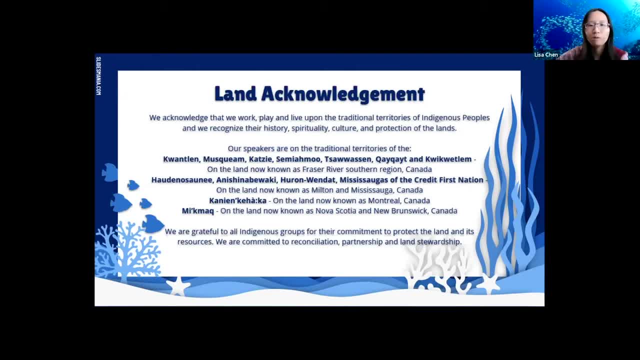 Canadian culture and history. When the European settlers arrived in Canada, they signed treaties with our Indigenous communities, but the Indigenous people did not surrender their land, Hence they are unceded territories. You will find throughout our presentation today. Indigenous voices are an important part of our decision-making process. 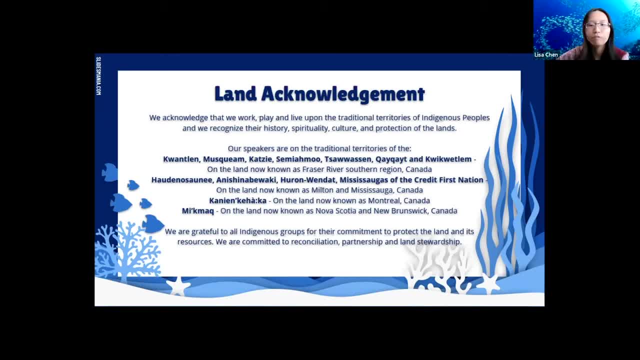 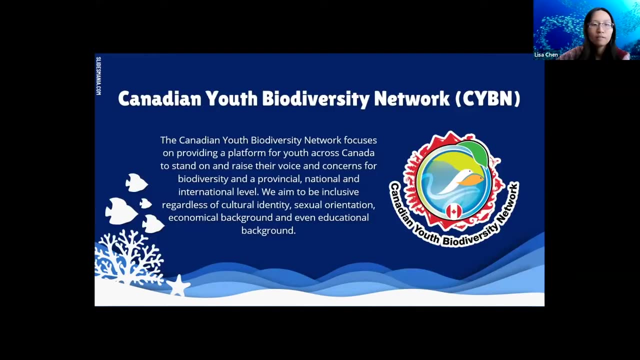 After all, how can we achieve marine conservation without first recognizing and respecting the importance of our Indigenous culture, knowledge, practices? And now I will pass on to Laura to give an introduction. Hello everyone. So the Canadian Youth Biodiversity Network first began in Montreal at one of the 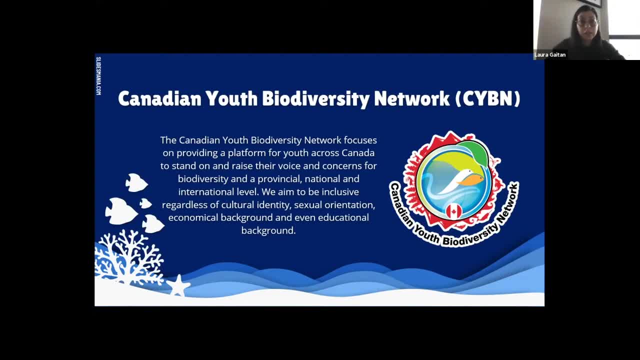 international meetings for the Convention on Biological Diversity, Canadian youth representatives met some of the amazing young people from the Global Youth Biodiversity Network. They encouraged them to start a Canadian chapter. So fast forward to today. the Canadian Youth Biodiversity Network is a global youth platform that features a broad range of 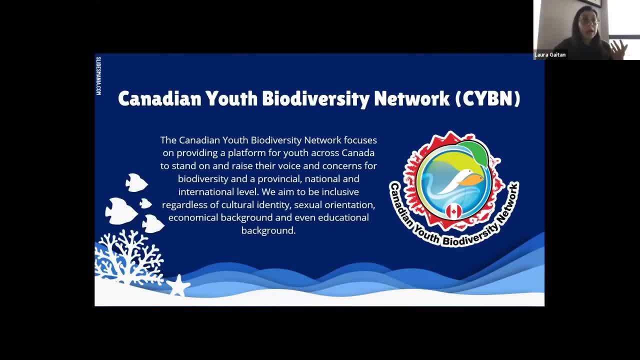 awareness-based activities to help youth in Canada to improve their understanding of the world. We have a national and international community of people in Canada and we have a community of indigenous people in Canada. We aim to be inclusive regardless of cultural identity, sexual orientation, economic and educational background. Some of the work we do includes: 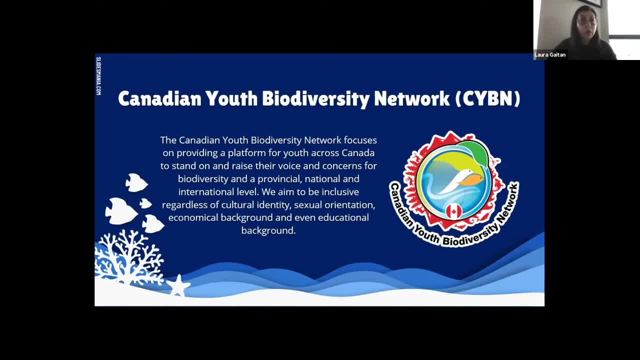 raising awareness through social media, providing educational webinars and building a network across Overall. with our work, we hope we can create a meaningful impact on our communities where we live in harmony with nature, now and for future generations. Thank you so much for coming to this. 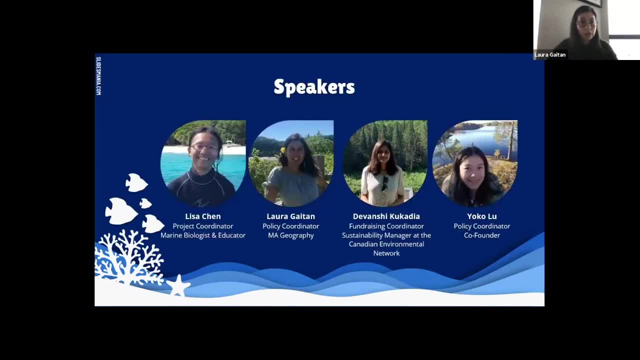 workshop on ocean conservation. So the speakers is: Lisa Chen, who is a Project Coordinator, and Marine Biologist and Educator, Devanshi Kukadia, who is a Fundraising Coordinator and Sustainability Manager at the Canadian Environmental Network. Joko Liu, who is a Policy Coordinator and a 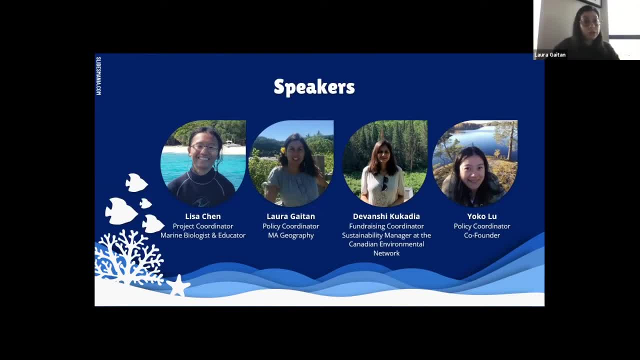 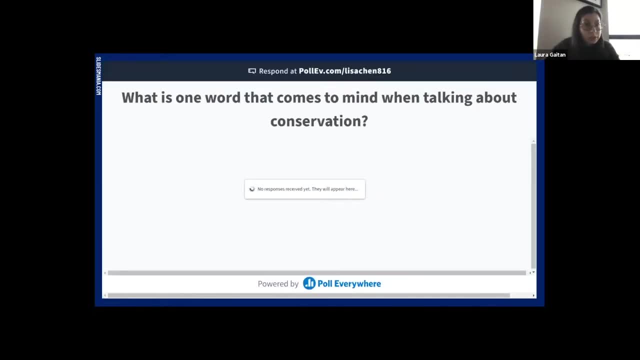 Co-Founder for CIVEN and myself, who I'm a Policy Coordinator and I'm finishing my MA in Geography. Next slide, please. So please, go to the poll, where we are going to ask you what is a word that comes to mind while talking about conservation. 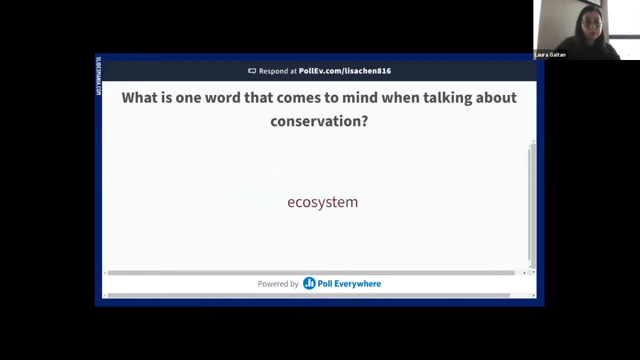 Thank you. We dropped the poll on the chat. Thank you. Wow, I see many interesting points that's coming up into our word cloud. Many of you agree that biodiversity is very important when we are talking about conservation, And some of you mentioned livelihood. that is something actually that we are going to talk about. that we cannot. 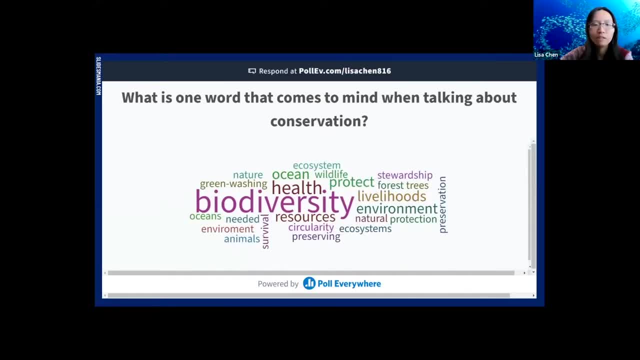 achieve conservation or sustainability without adjusting people's need and their livelihoods. We also have some questions for you in the chat. Okay, let me just unmute you to look at your questions so we can get them into the chat. Alright, I'm ready to go. 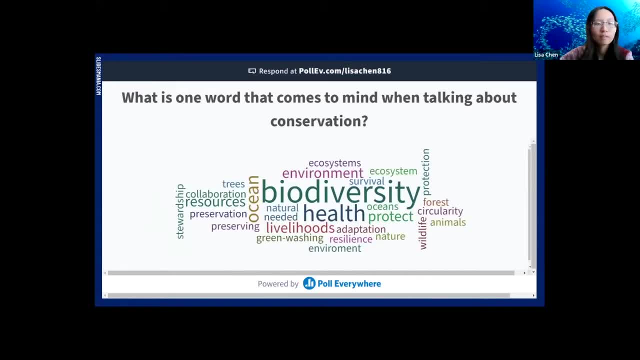 So you can answer any questions you'd like. Thank you, I think. I think. I think I'm more willing to try to hear your thoughts and your thoughts If you could just dig right into the chat, because it will help me understand your question. 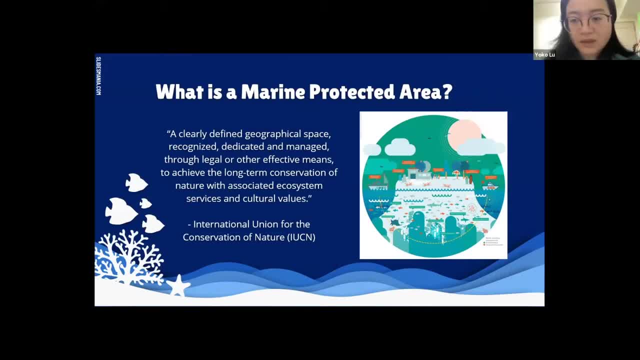 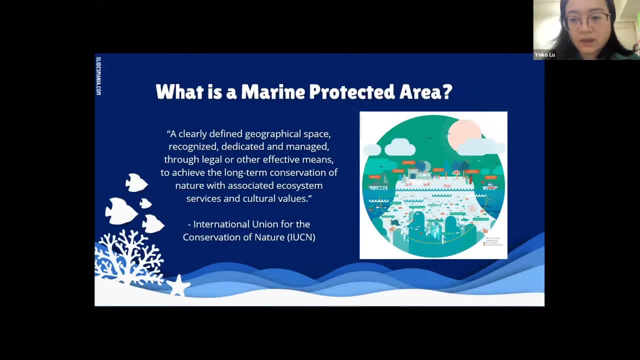 Thank you. conservation marine protect area comes to mind. In NPA, also known as the marine protect area, it's defined as a clearly defined geographical space, recognized, dedicated, managed through legal or other effective means to achieve the long-term conservation of nature. 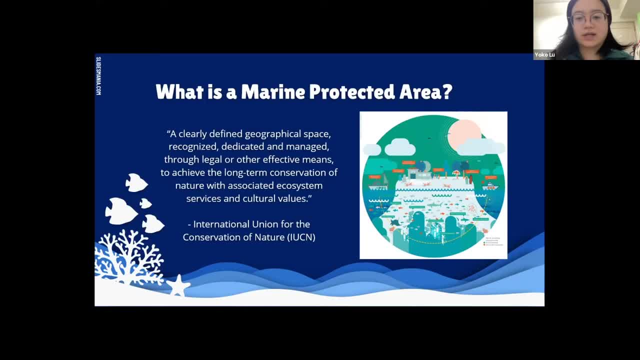 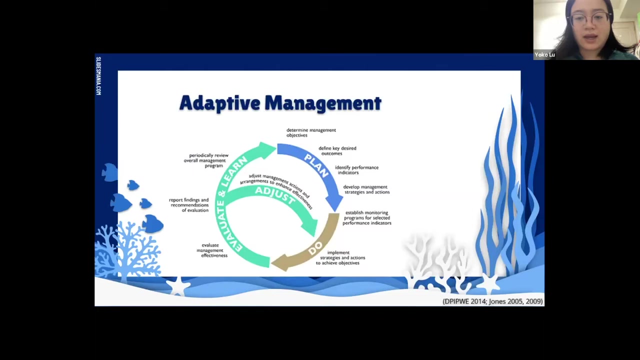 with associated ecosystem services and cultural values, as defined by the IUCN. I want to highlight that, according to this definition, NPA does not only conserve nature, but it also conserves cultural services. Adaptive management is something that happens in a five-year circle. 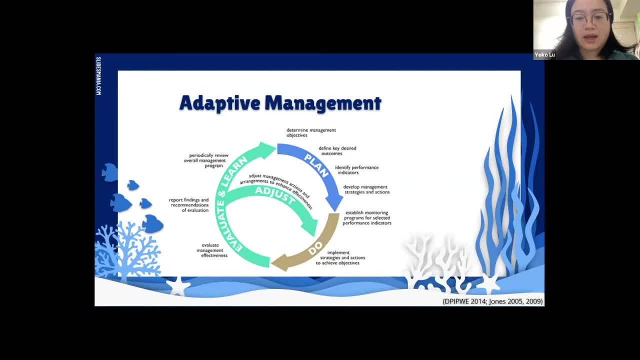 where, every five years, the NPA's review adjusted according to this graph. As mentioned before, it is not enough to simply establish a park and therefore this adaptive management is needed to review the protected areas management scheme to see whether it's effective or not. 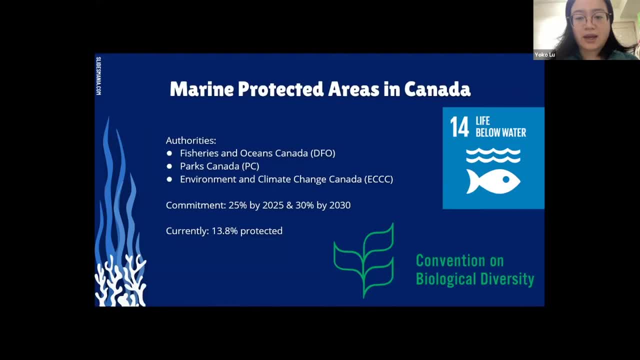 In Canada, there are three different governing bodies that have the power to make NPAs. however, they all have different mandates for the protected areas. Areas established under the fisheries and oceans Canada's Oceans Act are for the conservation of marine species, habitats, ecosystems, while 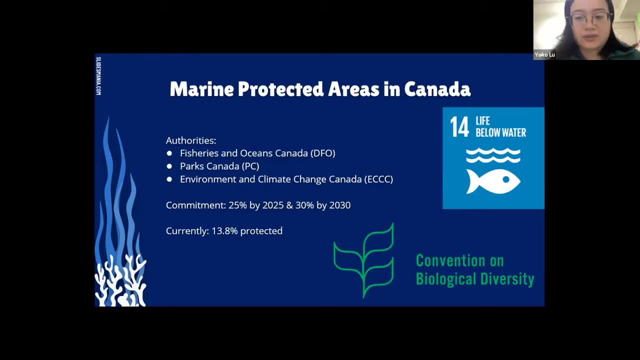 Parks Canada creates protected areas for the benefit, education- oh sorry, so the Oceans Act for the conservation of marine species, habitats, ecosystem, while Parks Canada creates protected areas for the benefit, education and enjoyment of the people of Canada and. 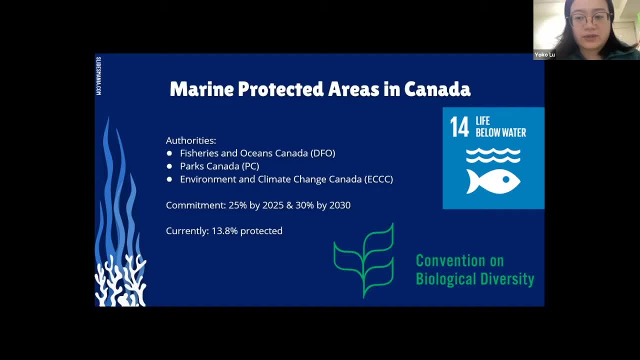 Environment and Climate Change. Canada aims to conserve habitat for a variety of wildlife, including migratory birds and endangered species. Canada is committed to protecting 25% of its marine waters by 2025 and 30% by 2013.. This aligns with the United Nations Sustainable Goals for Living and Life-Bearing Water and. 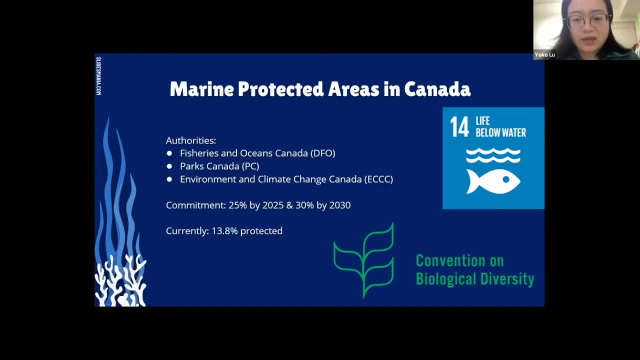 Aichi Target 11 from the Convention on Biological Diversity. Currently, about 30.8% of Canada's water is protected, compared to a global protected area coverage of 7.73%. This shows that Canada is doing a great effort in managing its waters. 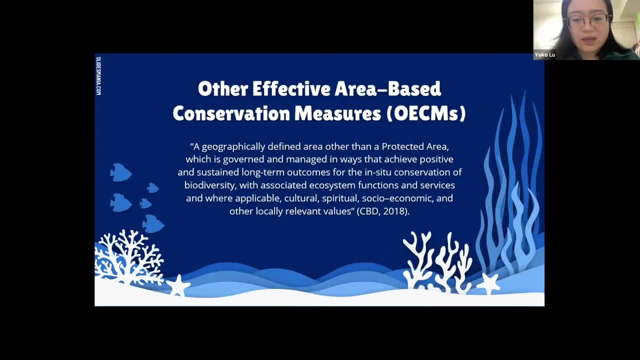 It is worth noting that these 30.8% protected areas are not created by the Oceans Act. They are not protected by the Oceans Act. Canada is committed to protecting these protected areas. This aligns with the United Nations Sustainable Goals for Living and Life-Bearing Water and. 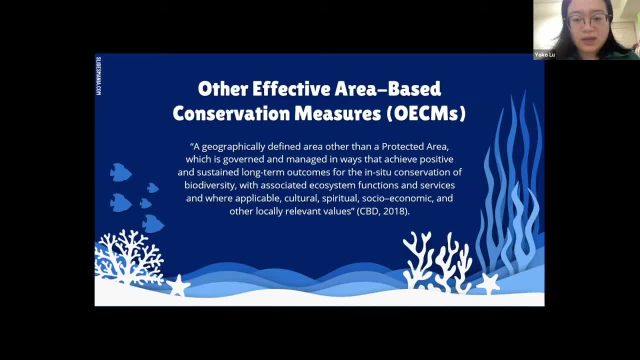 Aichi Target 11 from the Convention on Biological Diversity. Canada is committed to protecting these protected areas by 2030 and 2026.. This is why thisроal wide dl is supported under the designation of NPA, Due to the stakeholder consultation and adaptive management process. MPAs take a long time to 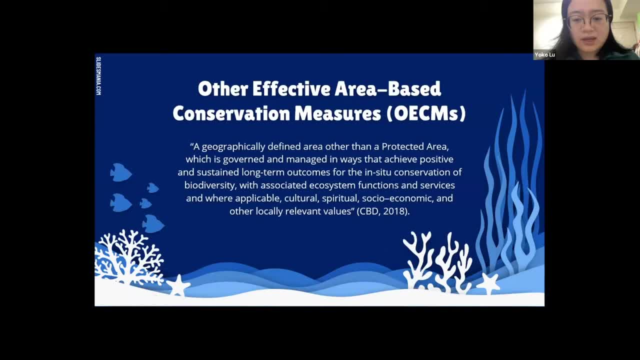 establish and a lot of resources to manage. Therefore, the Convention on Biological Diversity created the conservation designation known as Other Affected Area Based Conservation Measures, which is a geographically different area, other than a protected area, which is governed and managed in ways that achieve positive and sustained long-term outcomes. 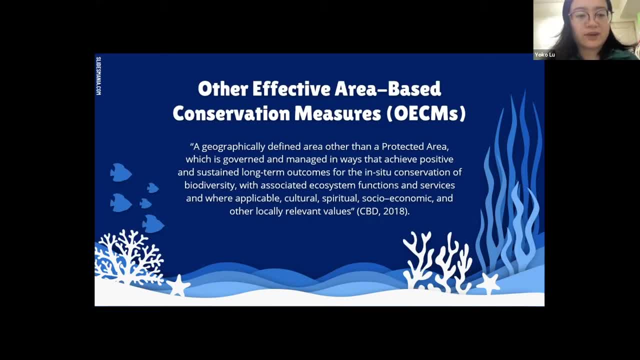 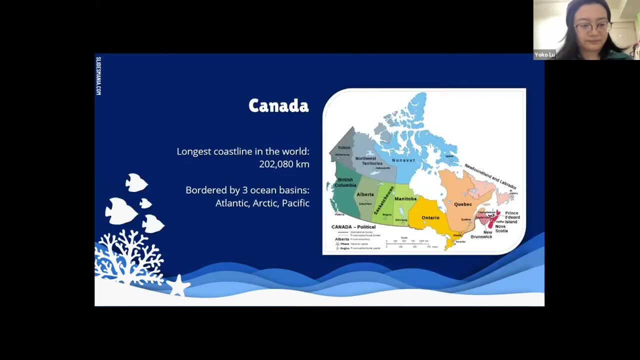 for the in-situ conservation of biodiversity, with associated ecosystem functions and services and, where applicable, cultural, spiritual, socioeconomic and other locally relevant values. Now, moving on to Canadian marine geography, Canada has the longest coastline of the world, As you can see on our slide. it is actually 3.7 times longer than the second longest coastline of Indonesia. 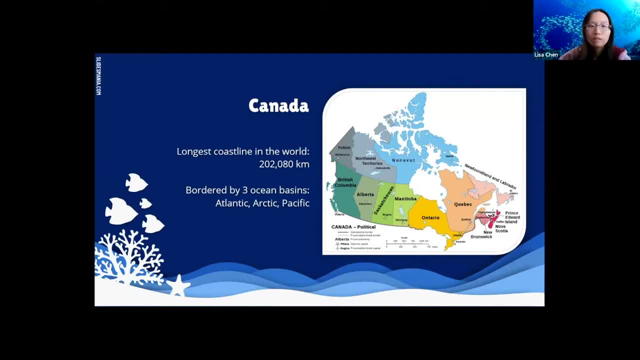 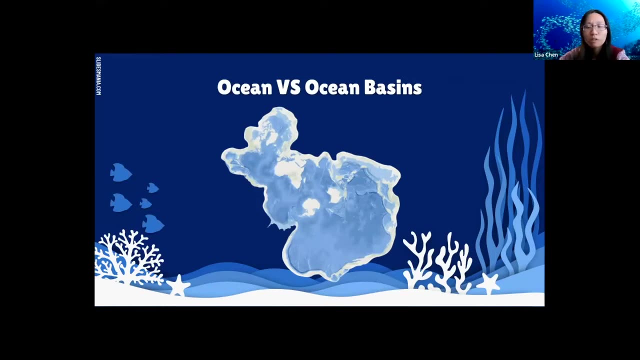 Canada borders three ocean basins, which are the Atlantic, the Arctic and the Pacific. Now, the emphasis here is on ocean basins and not oceans, because, as you can see on this map, we actually only have one big global ocean. All the ocean basins are connected to each other and, if we mistake, 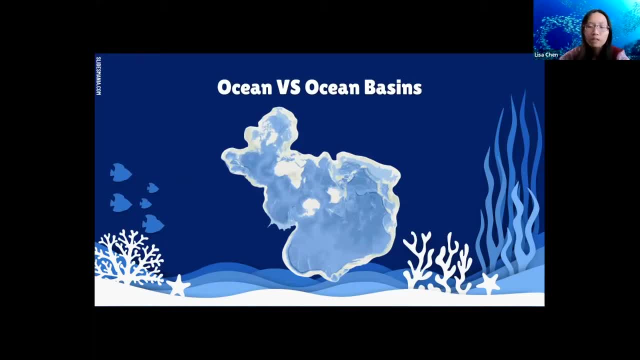 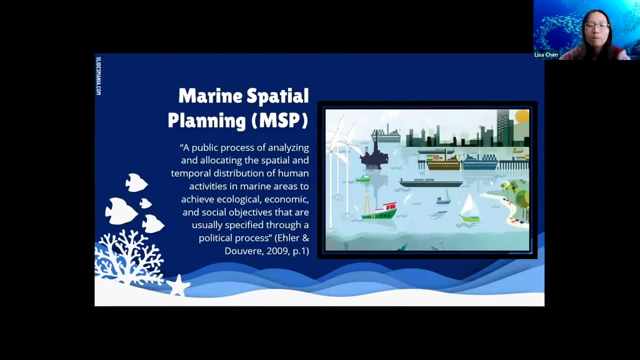 and we label ocean basins as oceans, we are undermining the urgency and the need for global marine conservation efforts. Now we can talk about marine protection and sustainability without talking about marine spatial planning or MSP. MSP is defined as a popular process of analyzing and allocating the spatial and temporal distribution of human activities in marine areas to achieve ecological, economic and social objectives. 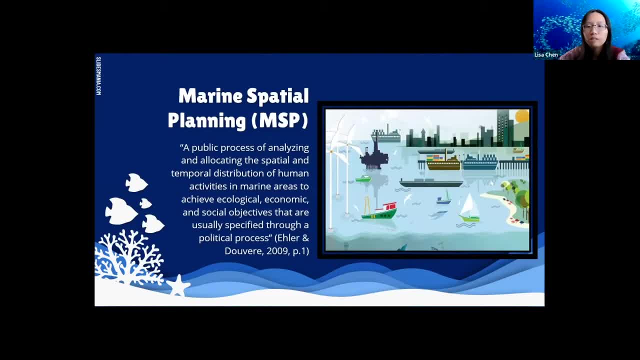 that are usury. specific through a protesters that are UC. specific through a political process. This means that environmental protection measures must balance with socio-economic and cultural needs of humans in order to be sustainable, because otherwise you will get very little compliance to the protection measures and create paper parties. 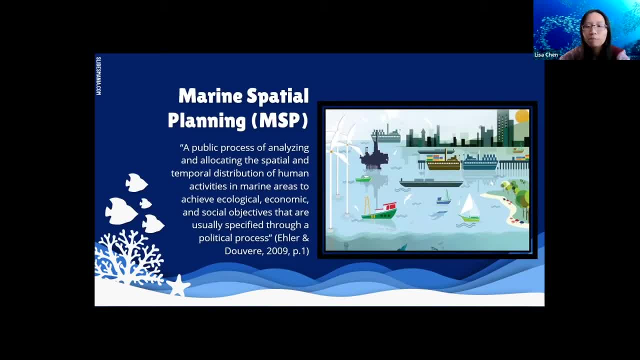 Finally, the political processes emphasize the importance of public consultation and having all stakeholders at the table to ensure that research is a sustainable process- Two belts To integrate that context and to discuss that with the communities. supporting plan is acceptable to everyone, Compared to traditional sectoral management where individual sectors manage their own. 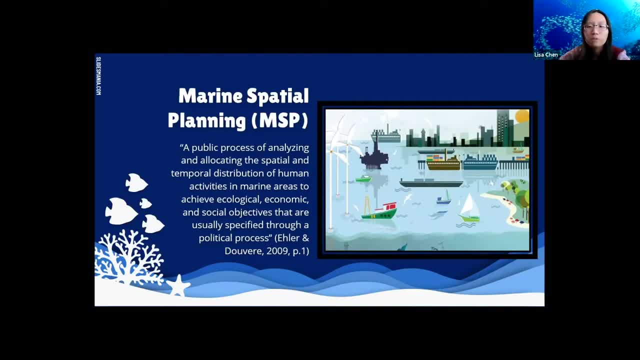 uses of the marine space. MSP is integrated between sectors and levels of government, adapted to changing circumstances and participatory by actively involving stakeholders. By incorporating these concepts, MSP seeks to minimize conflicts between marine users and between users and the environment, And it is this concept that needs to be carried forward when establishing MPAs. 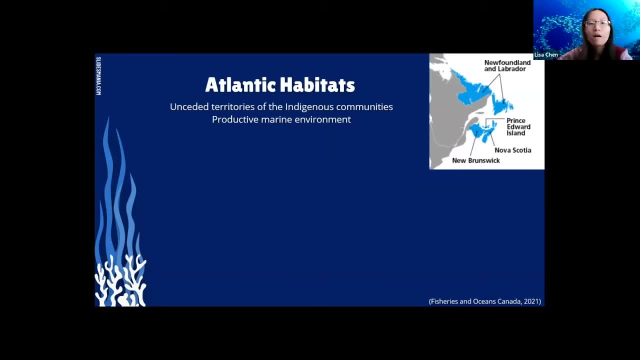 Moving on to the Atlantic coast of Canada, which includes four provinces, which are New Brunswick, Nova Scotia, Prince Edward Island and Newfoundland and Labrador. As I mentioned in my land acknowledgement, these provinces belong to the unseeded territory of our indigenous community. 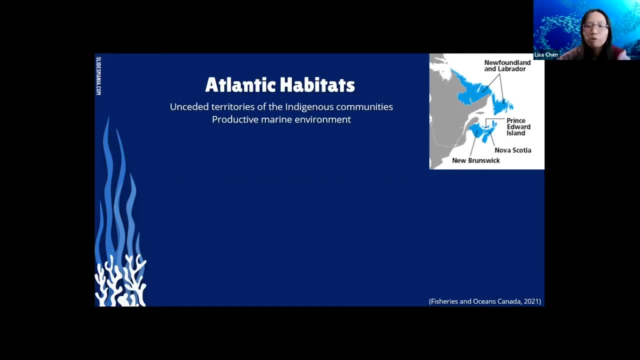 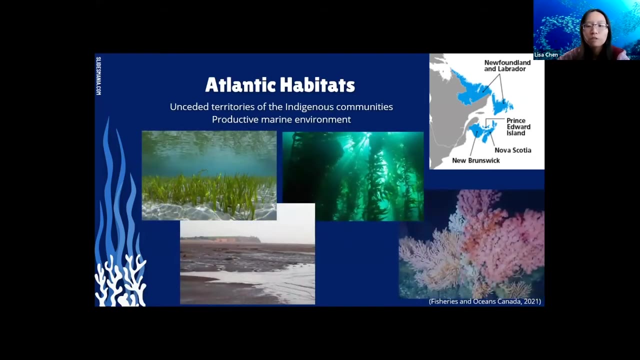 The waters of this coast. This is highly productive as the warm Gulf Gulf Stream from the south mixes with the cold Labrador current from the north, which brings a lot of nutrients for phytoplankton to grow and support our diverse number of marine habitats, which range from seagrass. 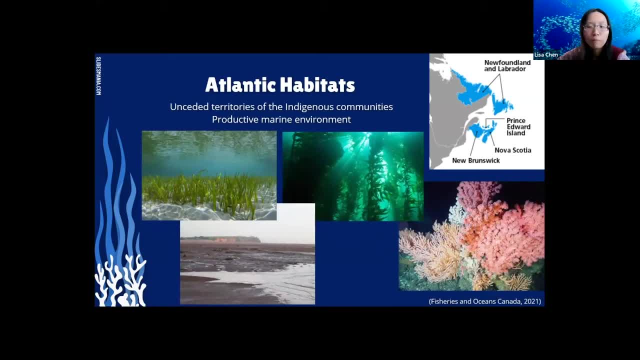 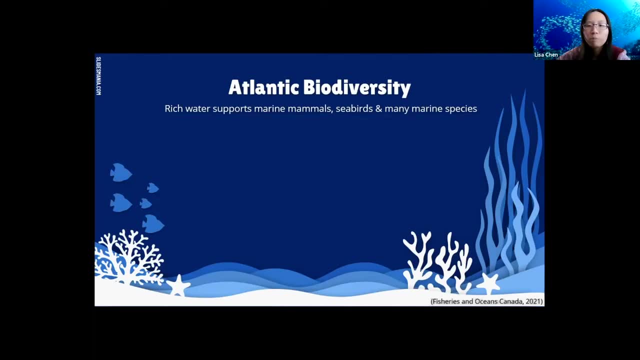 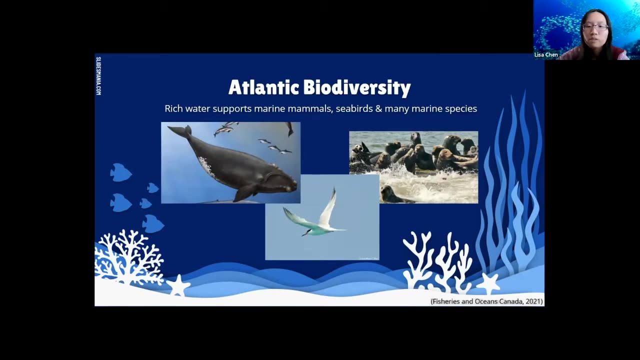 beds, to large expanses of mudflats, to cow beds and cold water corals. Due to the productive Atlantic water, it also supports a large window of marine mammals, such as whales, dolphins, seals and seabirds and other marine species. 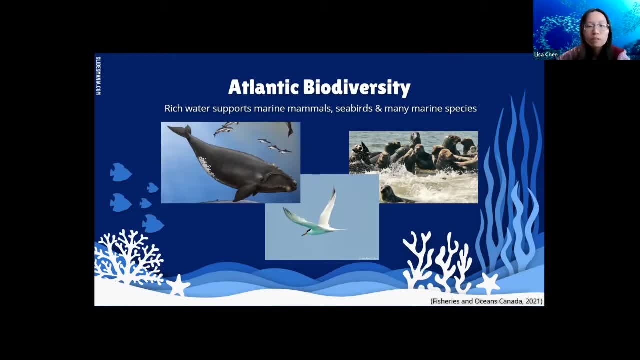 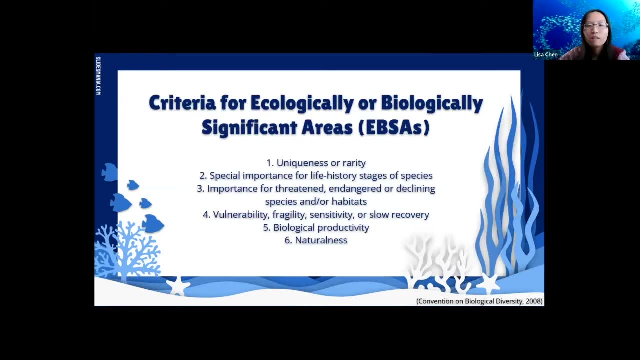 Our guest speakers will go into more depth on marine mammals and seabirds conservation. This productivity also makes it very difficult to identify ecologically and biologically significant areas, to create protected areas as different habitats, life stages of species and the uniqueness, importance, vulnerability. 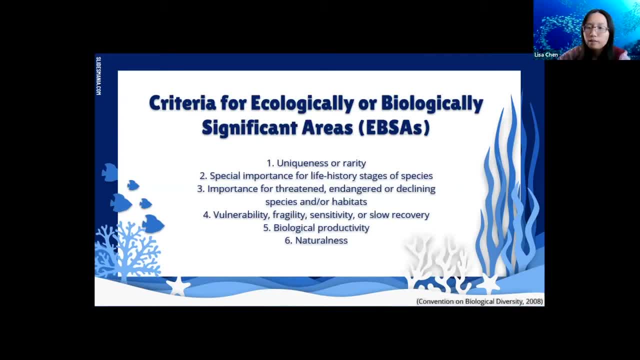 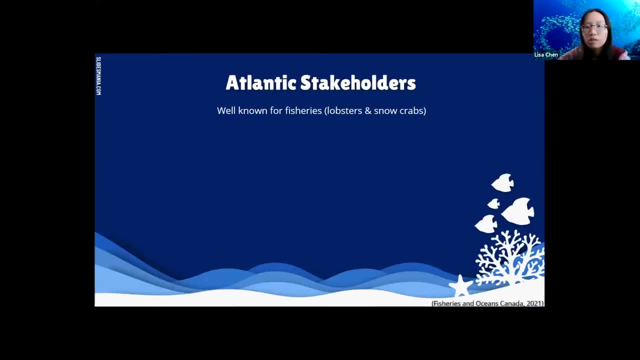 So, as I mentioned in my land acknowledgement, I would like to thank all of you. Thank you, Thank you. With that, I want to share with you the next agenda item and also get some thoughts from those in the community. Thank you, 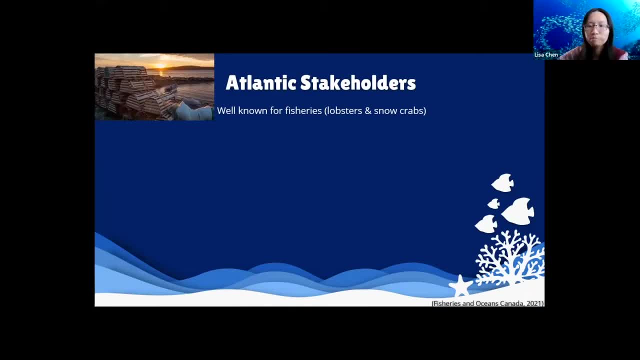 So yeah. So thisienda question is: what do my host? no waterwarrior groups need to think about. I didn t want to include the last point. Yeah, are also of great importance. According to our treaties, indigenous fishers have the right to a moderate livelihood fishery. 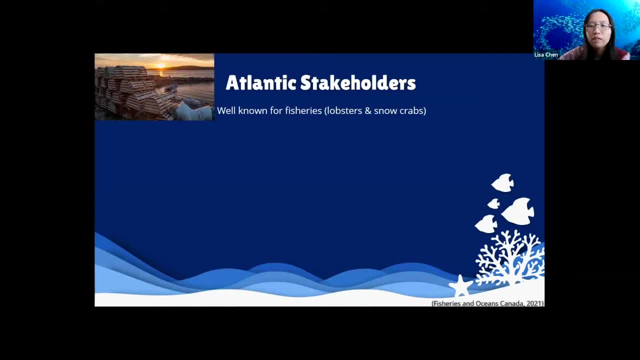 As we currently do not have a definition for moderate livelihood, this has created a contemporary conflict between fishers, government, local and non-governmental organizations. Further, the Atlantic also houses a number of marine and land-based aquaculture facilities. Our productive water also drives the industry. 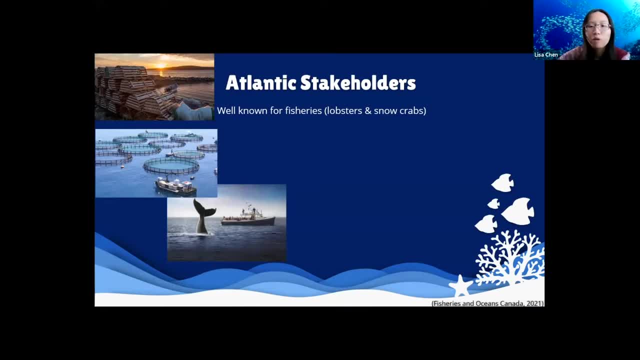 the tourism industry by welcoming tourists from around the world to come and well watch And, like many coastal areas, shipping, oil and gas explorations are ongoing. Finally, the Bay of Fundy area in the Atlantic region has the highest tides in the world. 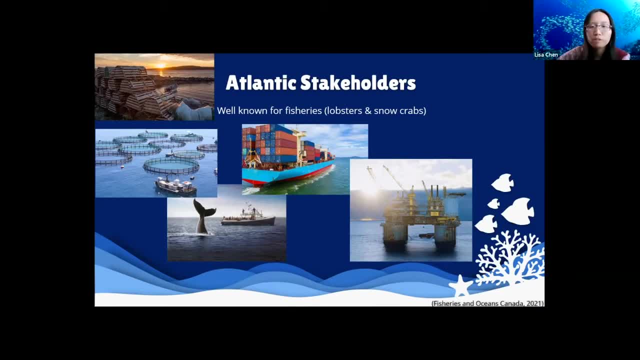 where there can be a tidal amplitude of as much of 16 meters between high and low tide, which offers an opportunity to develop renewable energy such as the tides. Therefore, marine protection in the Atlantic region must balance the environmental protection with cultural, socioeconomic and environmental needs. 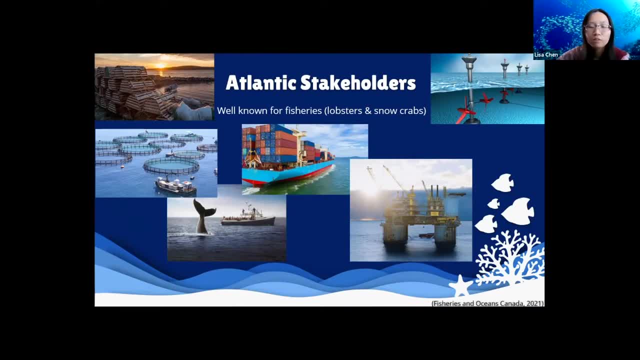 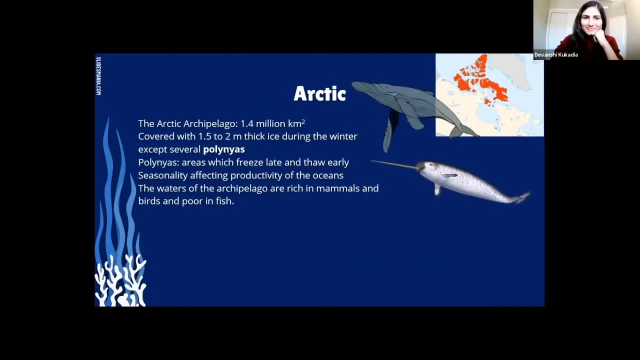 of all the stakeholders. Now I will pass on to Devanshu to tell us a little bit about the Arctic. Hi everyone, Let's take a trip to the Arctic Ocean. So Arctic archipelago is in Northern Canada and it occupies an area of 1.4 million square kilometers. 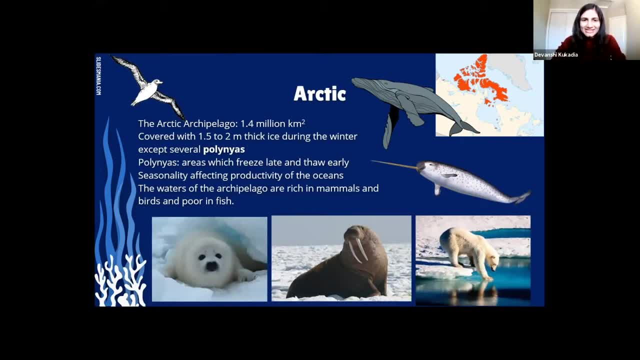 And it's formed by almost 36,563 small and large islands, And it is present in the three territories of Canada, namely the Northwest Territories and Yukon. Throughout the winter, the whole archipelago is covered with 1.5 to 2-meter thick ice. 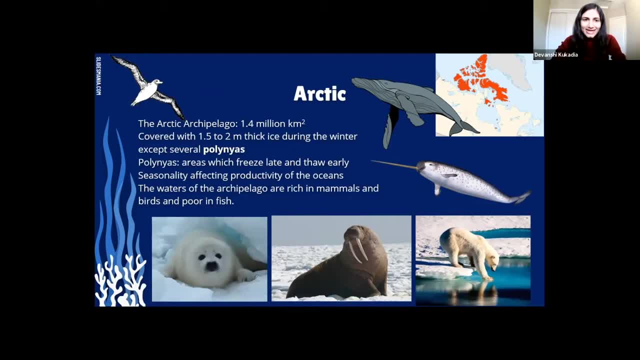 except for the polyneas. Now you may ask what polyneas? So polyneas are areas that freeze. Basically they freeze late and thaw early, So they are like open water zones when everything else is frozen, And that's why in winter it attracts. 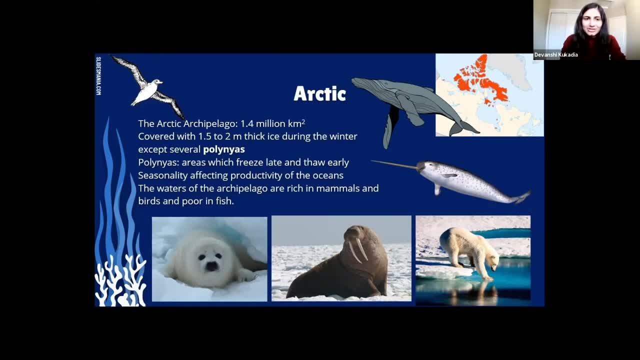 a lot of marine mammals, because marine mammals need to come to the surface to breathe. So if everything is frozen, they use the polyneas And in spring polyneas, so sunlight penetrates into the oceans through these polyneas, So they are frozen. 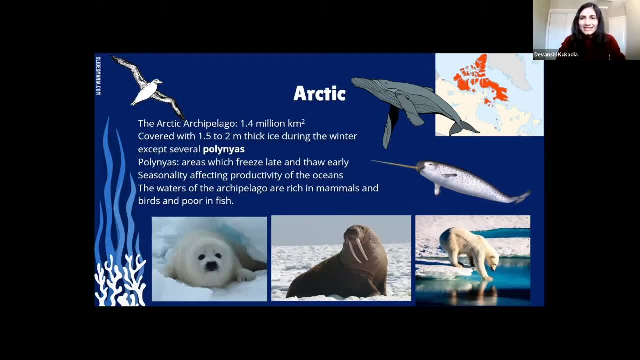 So it gives rise to like planktons And it increases the productivity of oceans. So seasonality affects the productivity of Arctic Ocean And the waters of this region are very rich in mammal species But they're quite poor in fish species. 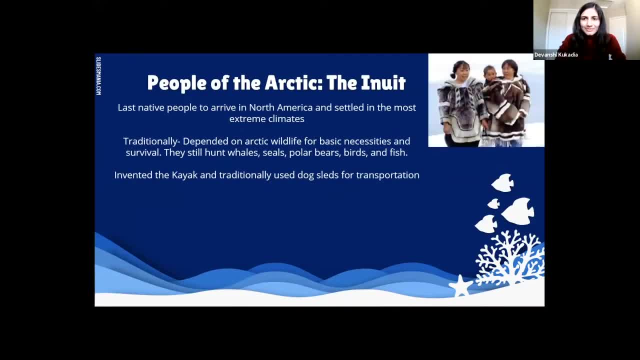 Next slide: Lisa, Yeah, So the Inuit people inhabit the Arctic. They were the last ones to settle, come and settle In North America And they occupied the harshest climates when everything else in the south of Arctic was occupied by other indigenous people. 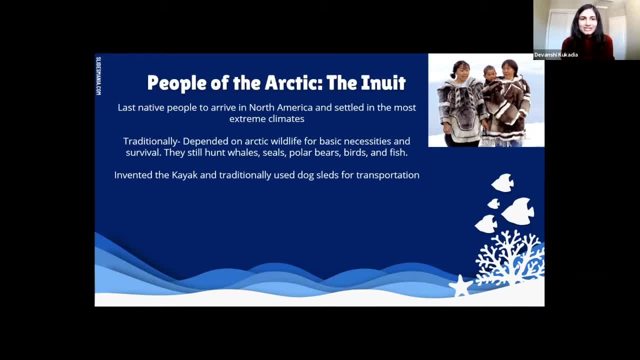 Traditionally, just because the weather is so harsh, it's so cold, that it's not possible to cultivate and grow like fruits and vegetables and food. So they depend on Arctic wildlife for their basic subsistence And even presently they still have like a lot of food. 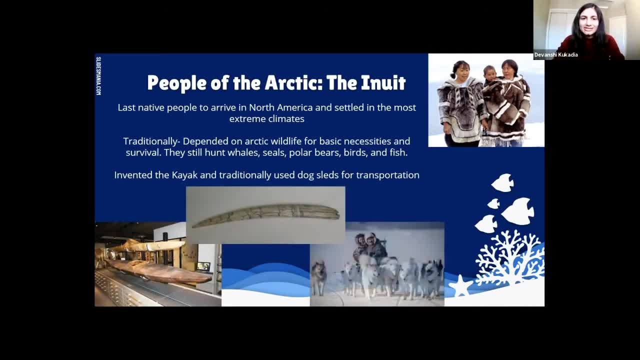 So they have a lot of food. So they have a lot of food. So they have a lot of food. They harvest whales, seals, polar bears for their consumption and to support their lives. They also invented kayaks, So traditionally they were made through seal skins. 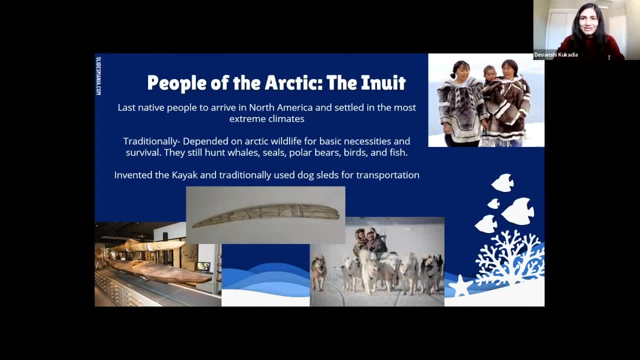 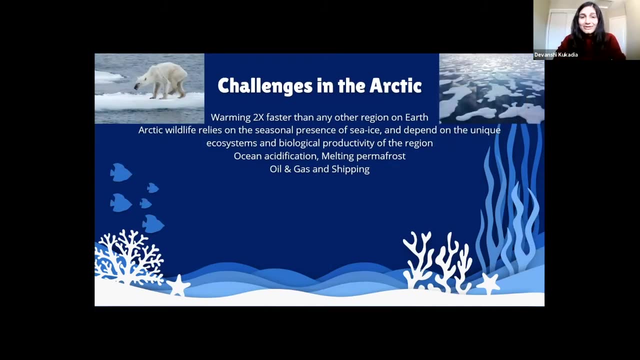 And they also use dog sleds for transportation on land and sea ice, because you cannot drive a car on the ice, mostly Next slide. Arctic Ocean also faces a lot of challenges. It's warming two times faster than any other region of the Earth. 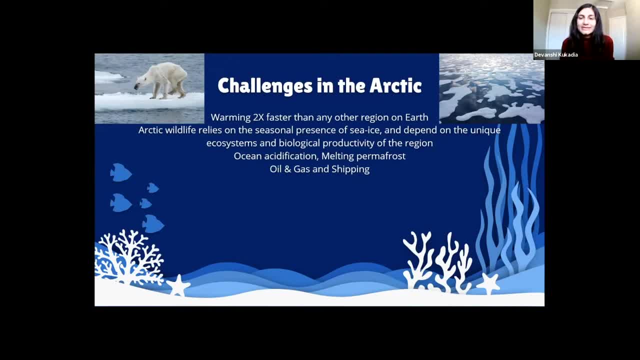 Because ice reflects the heat, but water absorbs the heat. So with melting ice, the water around the Arctic Ocean absorbs way more heat and it warms two times faster. Arctic wildlife relies on the sea ice to hunt and to survive in winter. 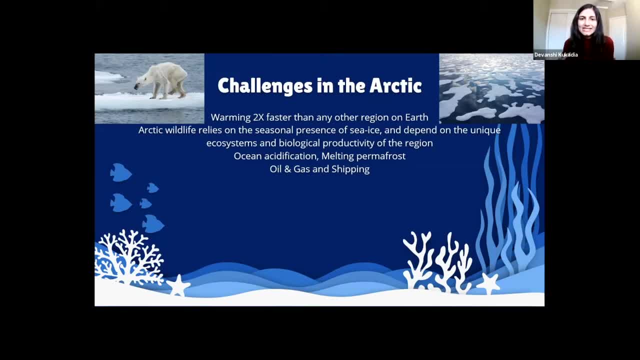 Like polar bears and walruses, they need ice patches on water to hunt. So they need ice patches on water to hunt and to survive. There is ocean acidification also. Just because there is higher carbon dioxide in the atmosphere, the ocean absorbs that carbon dioxide, which 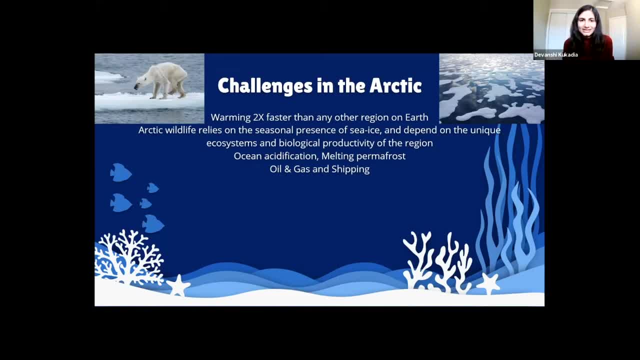 leads to increased acidity And it affects the shell formation process of the shellfishes, like crabs, mollusks et cetera, And it will lead to a catastrophic decline of the marine productivity. So also permafrost is melting. 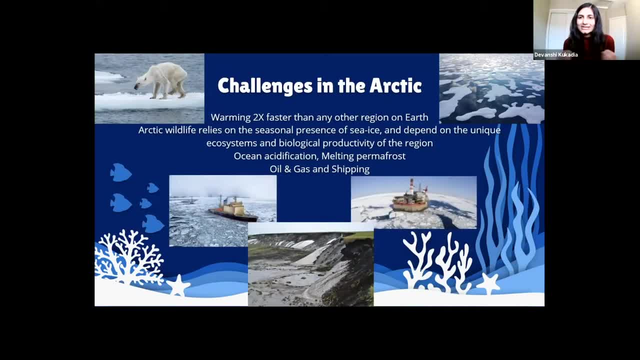 Now you might ask what permafrost is? It's soil, sand, rocks and ice together frozen in the land. It also has plant debris and stuff like that. So when the permafrost melts, all these plant debris starts decomposing and releases a lot of carbon dioxide. 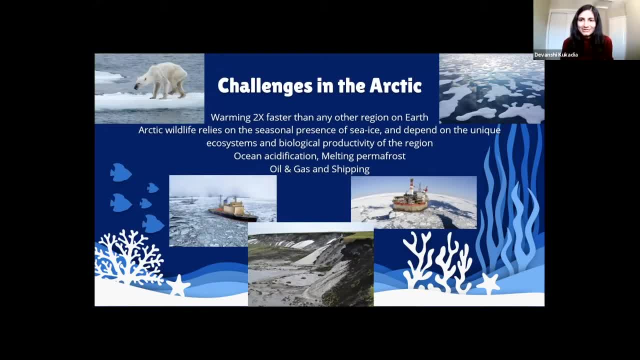 And to add to the issues, there's oil and gas exploration because of the melting of permafrost- Right Yeah, It's melting ice and it leads to oil spills. There is shipping, which leads to collision with mammals, and other issues in the Arctic. 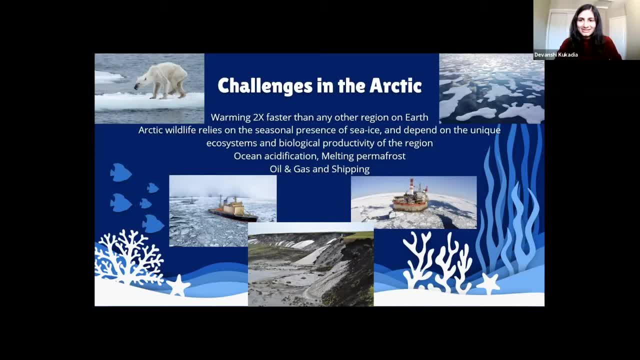 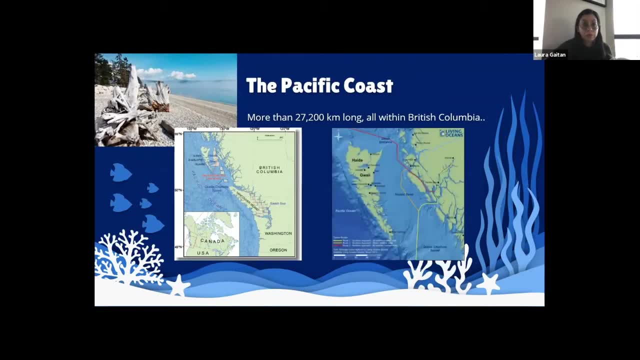 Now my colleague Laura will talk about the Pacific coast. Thanks. Thank you, Devanshi. So the Pacific coast is all within the province of British Columbia. The coastal landscape ranges from low-lying deltas to mountainous fjords. The coast is really an integral part of BC's economy. 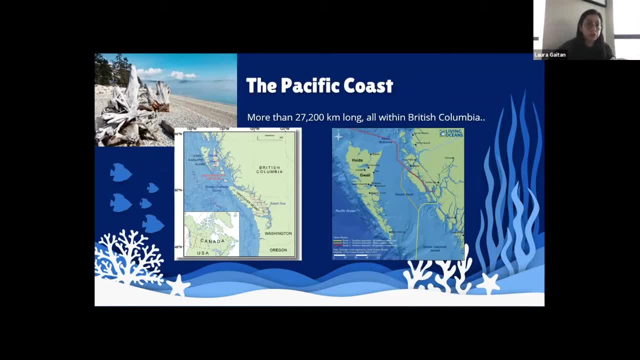 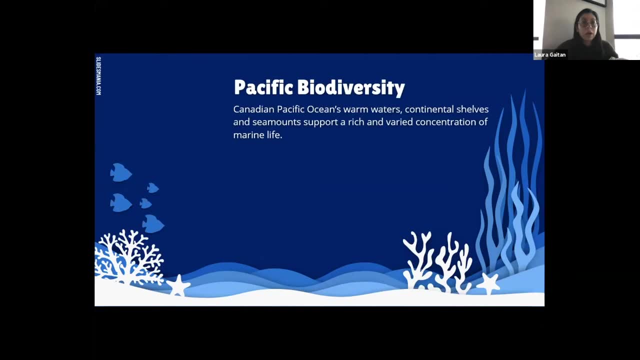 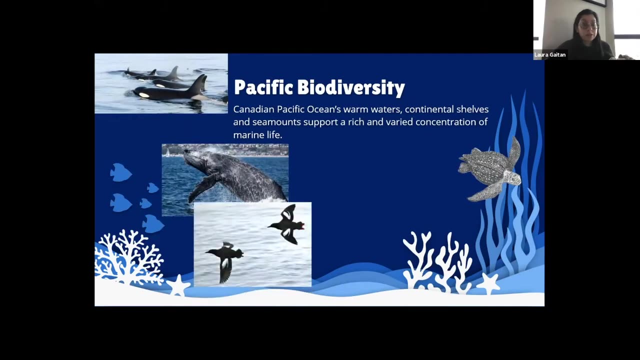 As many of the provinces, industry depend on the ocean. This include tourism, transportation, technology and seafood. So our Pacific Ocean supports a rich marine life. Species range from their very old, like now 9,000 year old, classes to very large like the blue whales. 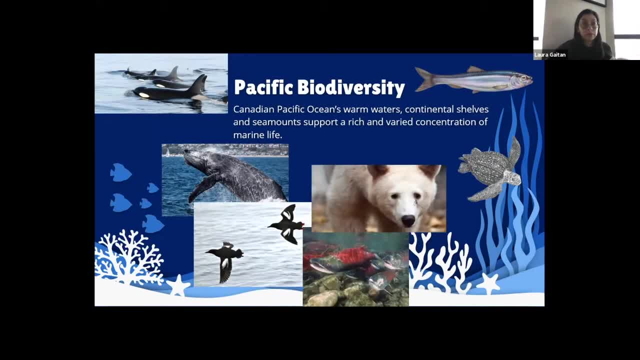 which is the largest animal, Other whales that live in this water, includes the humpback and killer whale. This area is also home to a large group of animals, such as range of marine birds, and, as for fish, the pacific herring is a foundation for more, for more, for most. 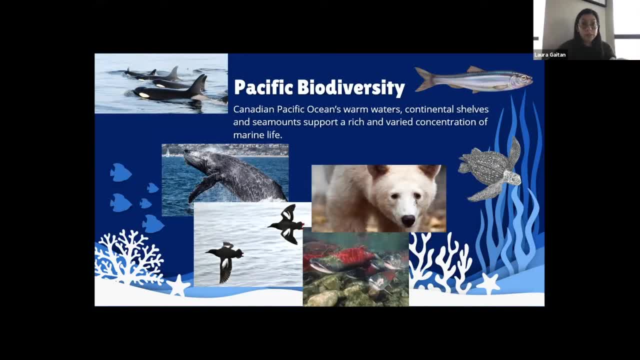 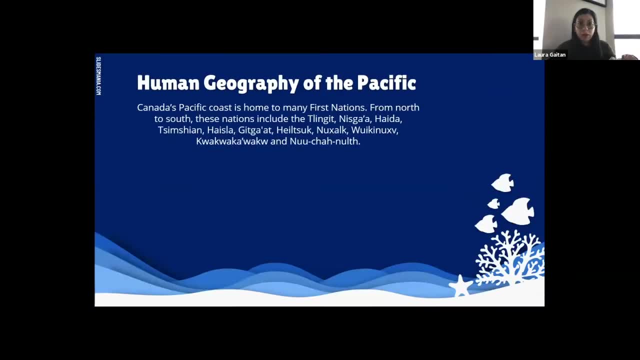 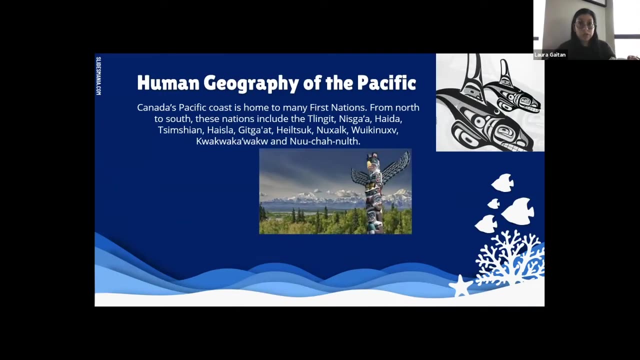 of the coastal food cycle and there's the salmon based ecosystem that stretches from the watersheds inland to the deep pacific. so the coast, our pacific coast, is home to many first nations. for thousands of years these coastal first nations have sophisticated fishing and sea. 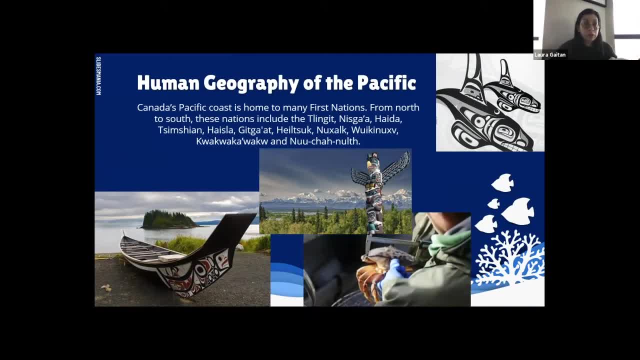 mammal hunting technology with river run salmon. it is a very important resource and a spiritual symbol. however, pacific salmon is facing multiple treats. this includes habitat destruction, pollution and unsustainable fishing practices. these threats increase with climate change, as salmon is very sensitive to high temperatures. so even a small increase in the warmth of the 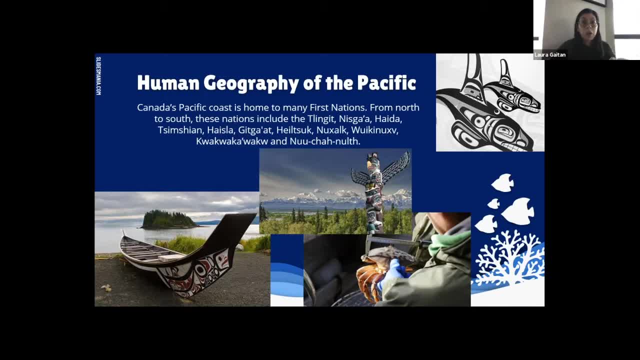 oceans and river can harm or kill them. when salmon populations are in danger, other members of the ecosystems are also threatened. for example, orca populations in the solid sea are decreasing the numbers. however, there is hope. many coastal first nations have signed a fisheries resource reconciliation agreement with the government of canada. 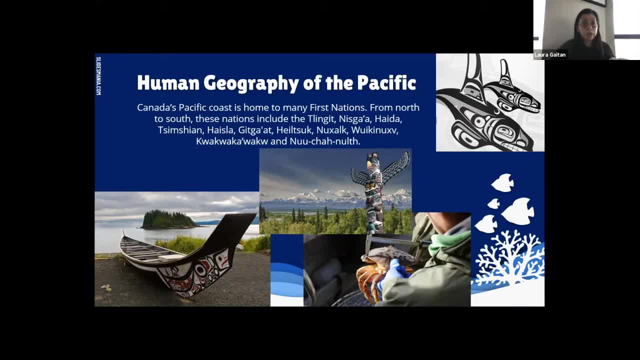 this agreement is facilitating an enhanced role in collaborative governance and in fisheries management and decision making processes for these coastal first nations. this legislation would support the organization of angus foals and spearhead Walt Narvik to become a partner of the four largest fishing communities in the world. 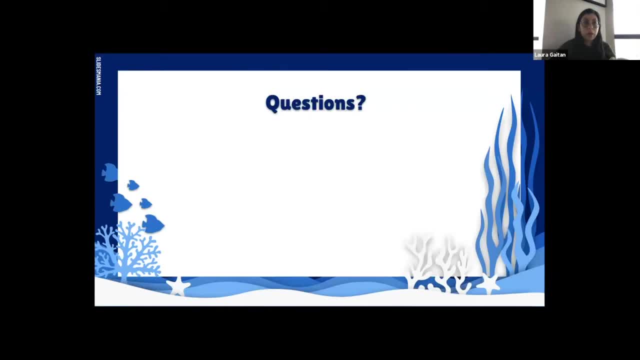 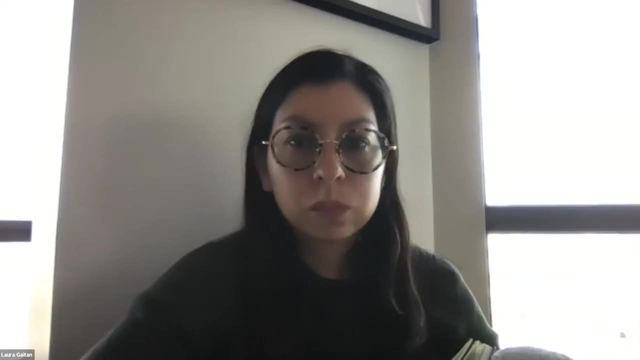 so this is a great opportunity to have a multi-day training on this weekend. so thank you to all the first nations whose territory make up of 40 percent of bc's coastal waters. thank you, next one, we wonder if you have any questions. you can drop them off the chat or just let us know. thank you. 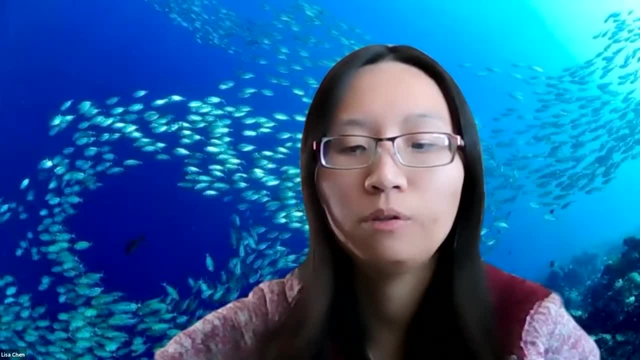 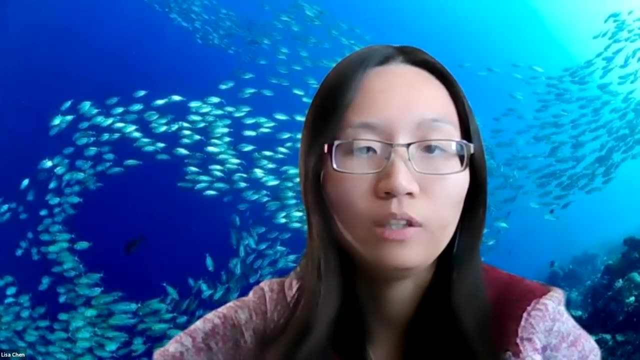 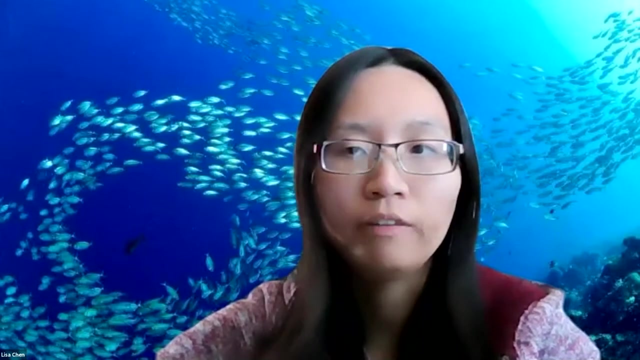 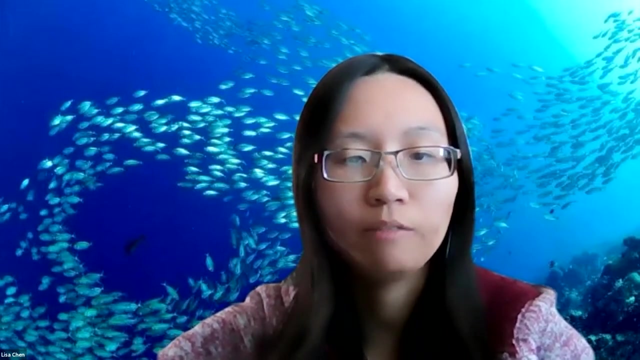 who are asking us what are some ways to include indigenous youth and other marginalized groups in water advocacy. This is actually an issue that's ongoing in Canada. There is an increase in recognition of indigenous ways of knowing and incorporating 2IC into our government system. 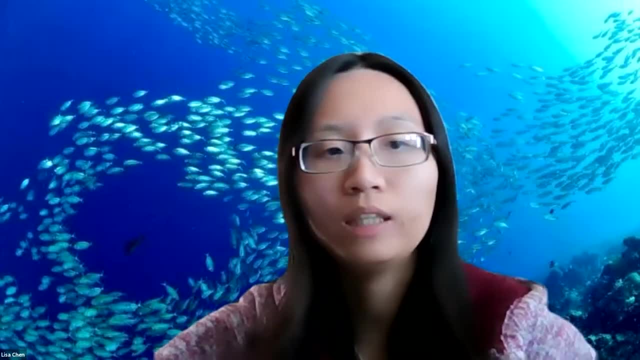 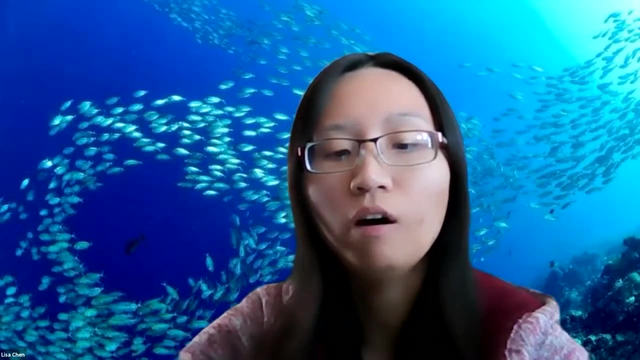 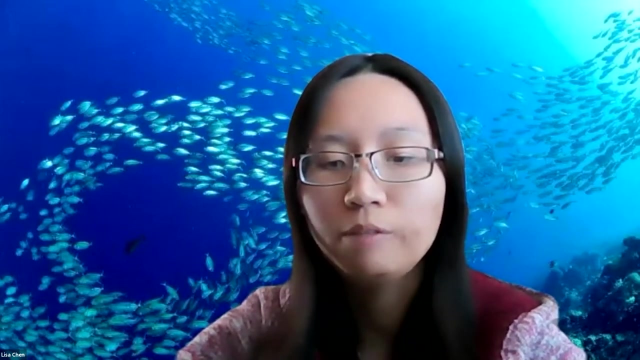 So 2IC includes that you are taking the goods and the strengths of the western knowledge system and the benefits of the indigenous knowledge system and combining them into a unique way to solve our environmental challenges, And I believe that is the way forward for other countries as. 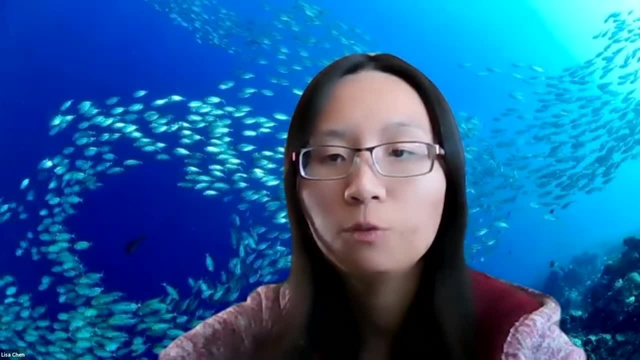 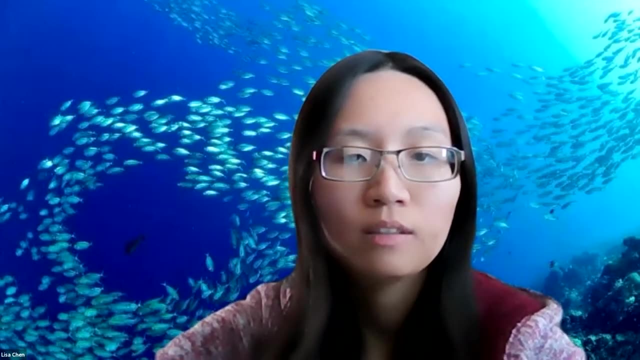 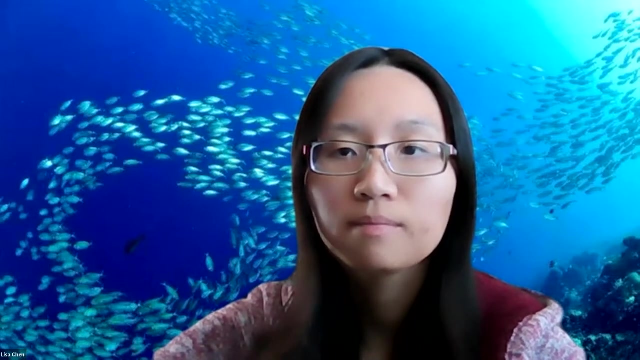 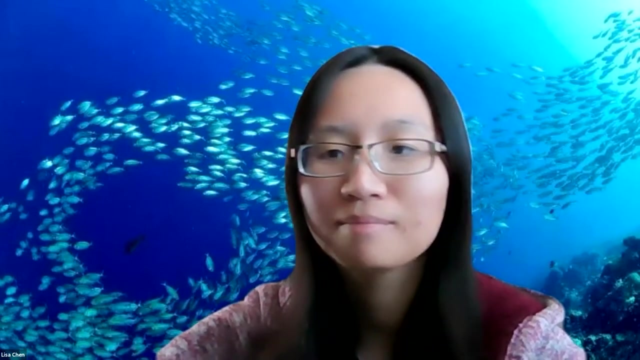 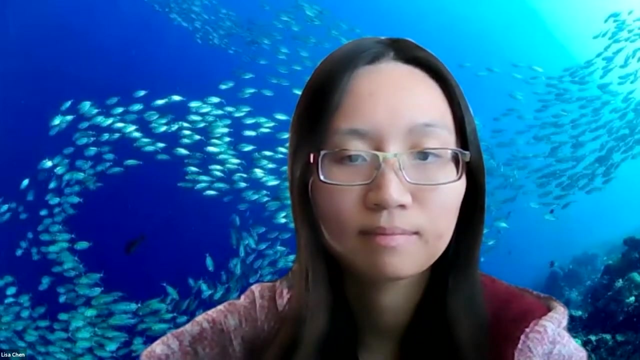 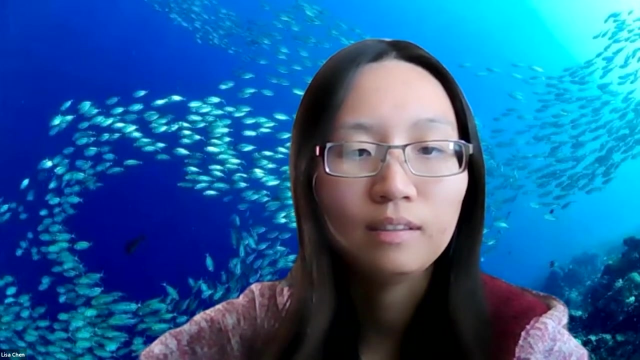 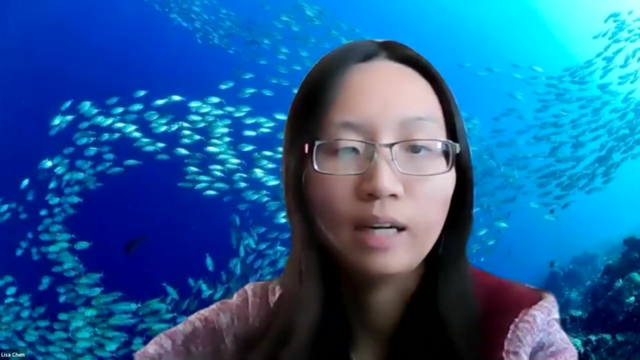 well as Canada to work on to continue doing wholesale research of conservation using 2Y-CN. Any other questions? If you have other questions later, you can drop them into the chat and we'll adjust them towards the end. So now perhaps we'll move on to our guest speakers. 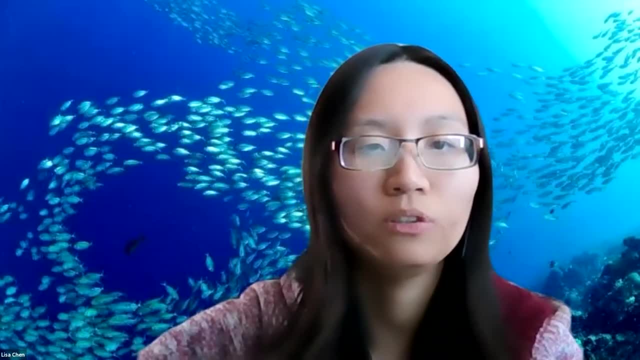 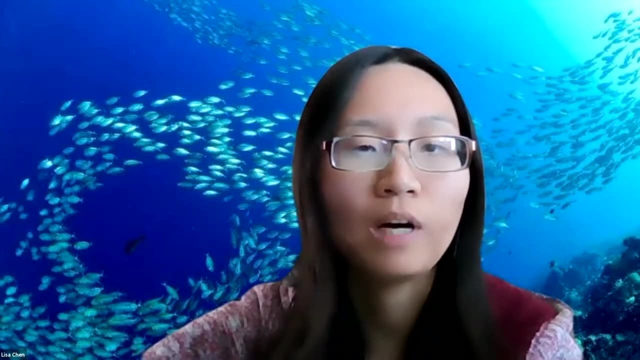 So first up, I would like to introduce Dr Hilary Morris-Murphy. She works at the Bethway Institution of Oceanography, which is part of the Ocean and Ecosystem Science Division at the Maritime Region of Fisheries and Oceans, Canada. 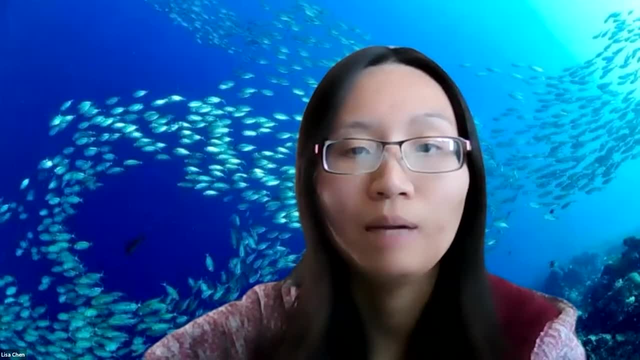 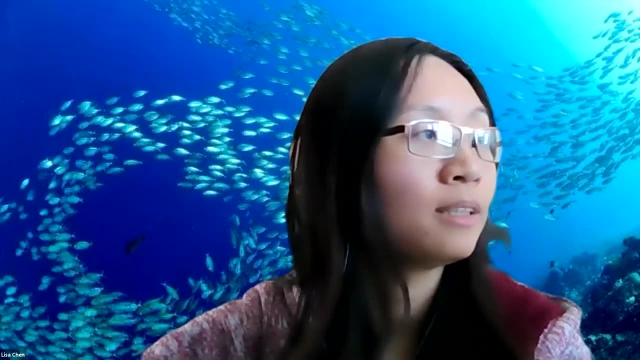 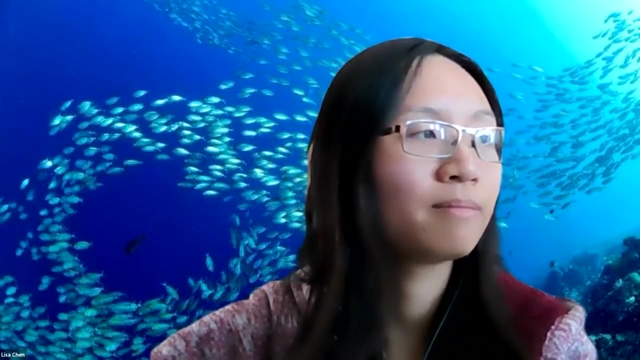 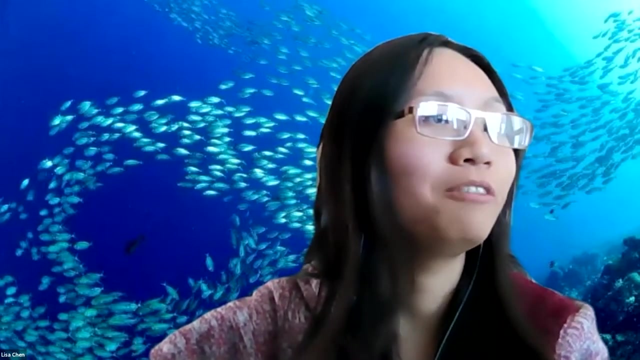 She works with whales and I believe she will talk about fisheries and oceans, Canada's role in management. So, Dr Hilary, you have the floor. Dr Hilary, you are muted right now. Okay, there we go. Thank you so much for the question. 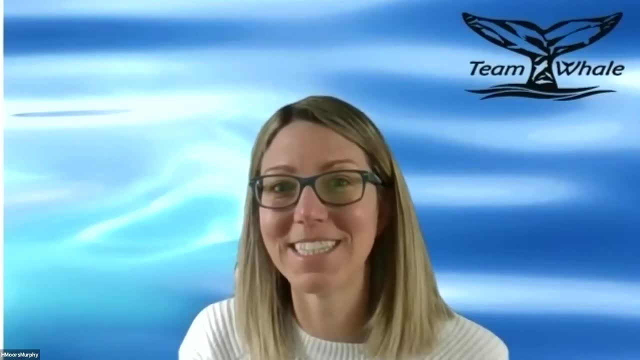 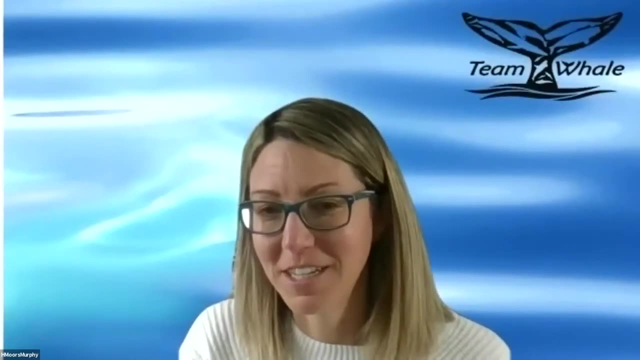 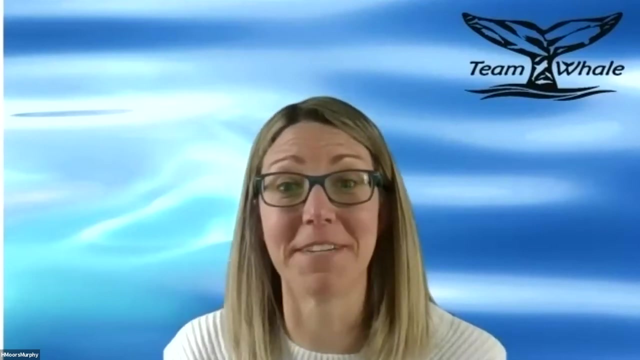 Thank you for the introduction. Can everyone hear me? Yes, Okay, excellent, I am going to shut off my video while I give my talk, just to reduce any bandwidth issues I may have, because I have a couple of videos that I do want to show. 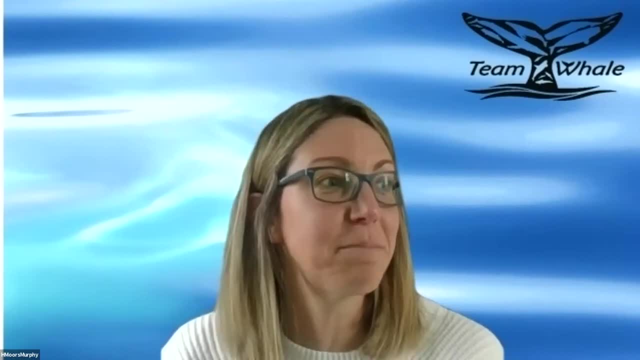 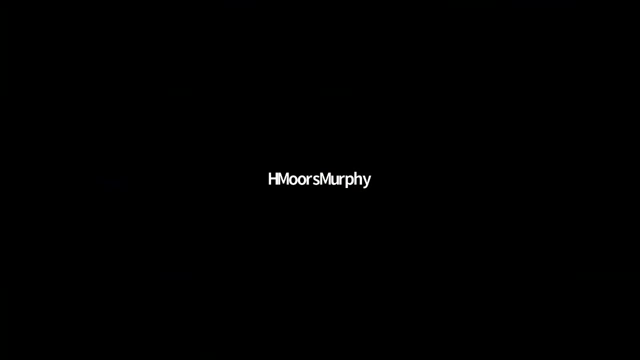 So I'm going to turn off my video here and get my PowerPoint up and running. Okay, Let's see here Share screen And I got to make sure I share my sound, So do you see my PowerPoint here? Yes, Excellent. 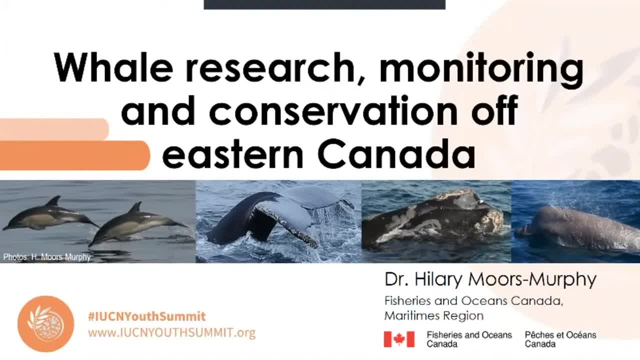 Well, hello everyone and thank you to the organizers so much for having me speak at this event. As mentioned, my name is Hilary Moores Murphy and I am a research scientist with Fisheries and Oceans, Canada in the Maritimes Region off the east coast of Canada, so around that Atlantic region that we saw. 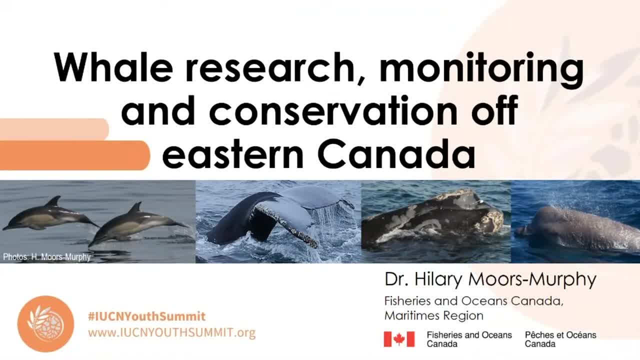 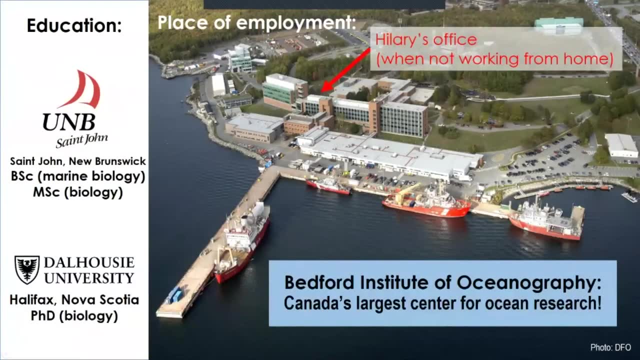 And I am excited to talk to you today about some of the whale research, monitoring and conservation me and my team are involved with within fisheries and oceans. But before I jump into things, just a couple of quick facts about me. So I did my Bachelor of Science and then my Masters of Science degree focused on seal acoustics, at the University of New Brunswick in St John, New Brunswick. 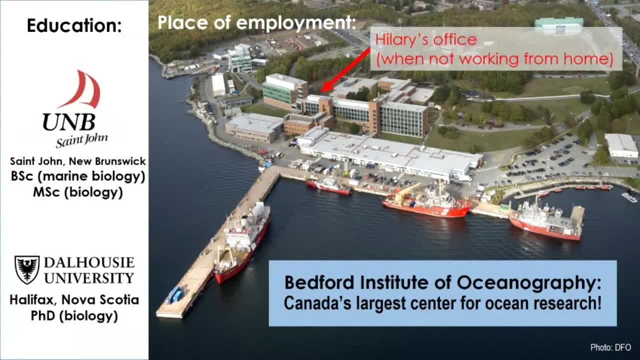 And then I did a PhD focused on cetacean or whale acoustics at Dalhousie University in Halifax, Nova Scotia, And I now work at the Bedford Institute of Oceanography, which is found in the Halifax area, And this is Canada's largest ocean research institute. 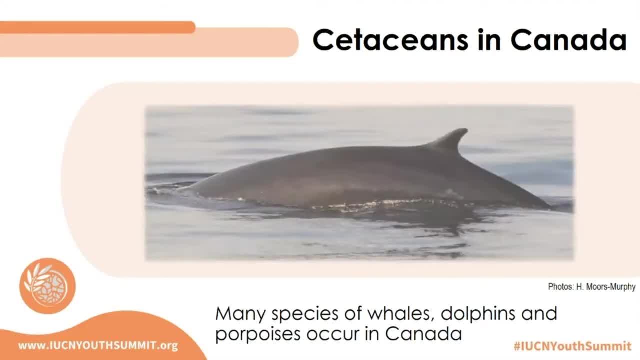 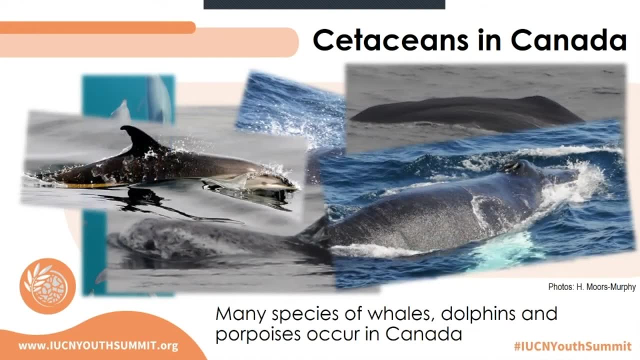 So it's a pretty cool place to work. Now, some of you may not know, but there are many different sources of oceanography. There are many different sources of oceanography. There are many different sources of oceanography. There are many different species of cetaceans. 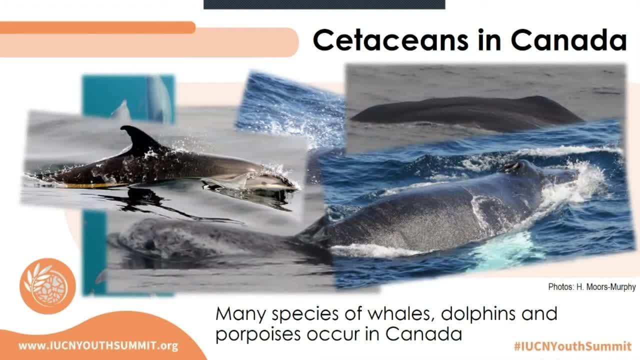 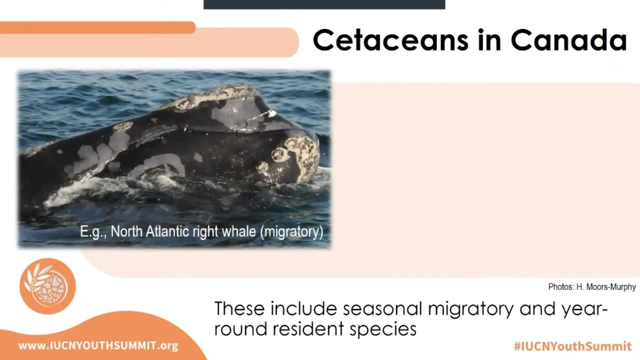 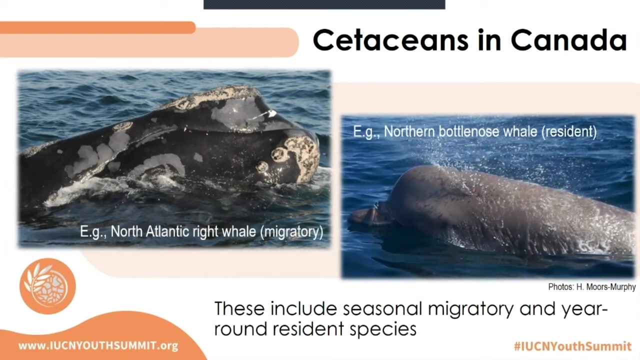 And cetaceans is really just a fancy word- meaning whales, dolphins and porpoises that occur in our Canadian waters And here off the east coast. we have more than 15 different commonly occurring species. These include seasonal migratory species such as the North Atlantic right whales, as well as year-round resident species like northern bottlenose whales. 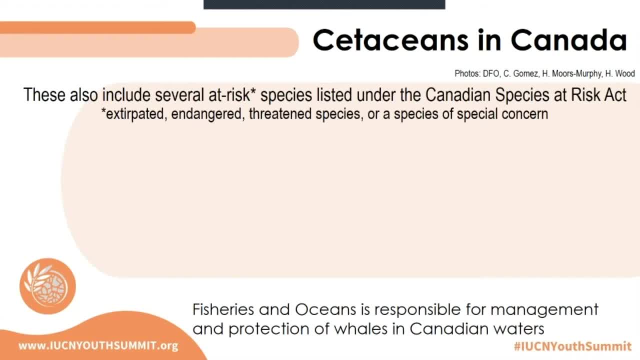 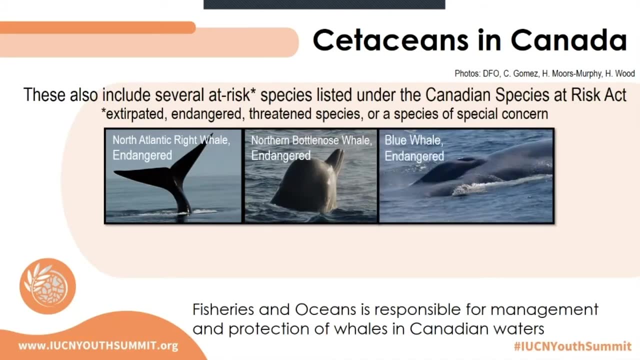 These also include several at-risk species or populations, In other words, endangered or threatened species or species of special concern, as recognized on Schedule 1 of our Canadian Species at Risk Act, And in many cases these species are also recognized as at-risk internationally, such as on the IUCN Red List of Threatened Species. 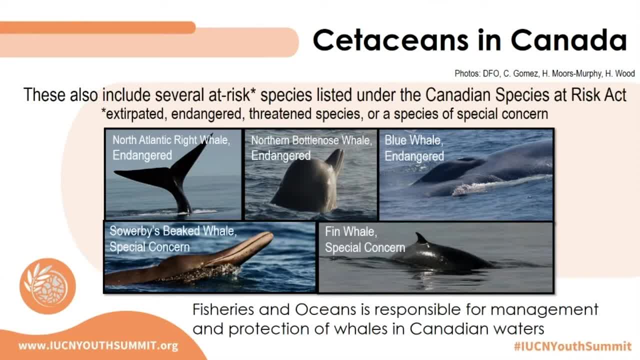 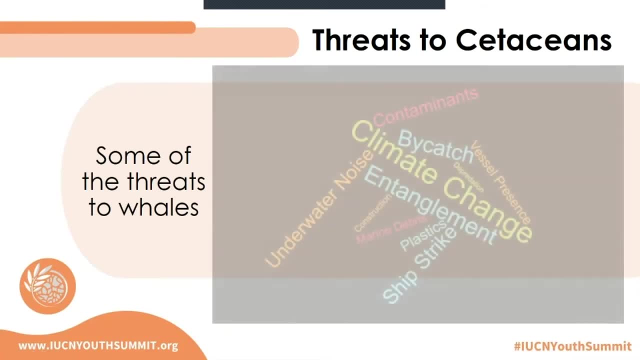 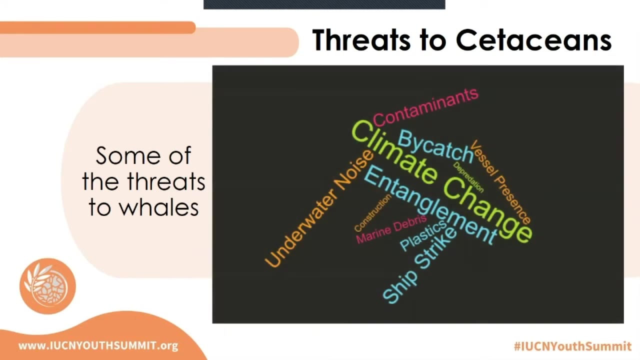 Fisheries and Oceans, Canada is responsible for the management and protection of whales in Canadian waters, Including these species here on the east coast listed under our Species at Risk Act. There are many different threats to whales and these are not unique to Canada: Climate change, entanglement, ship strikes, contaminants, pollution, underwater noise and much more. 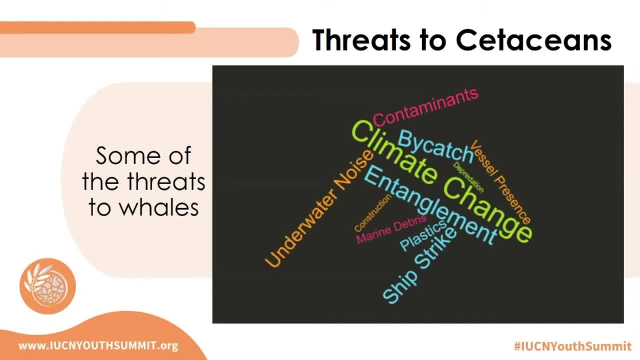 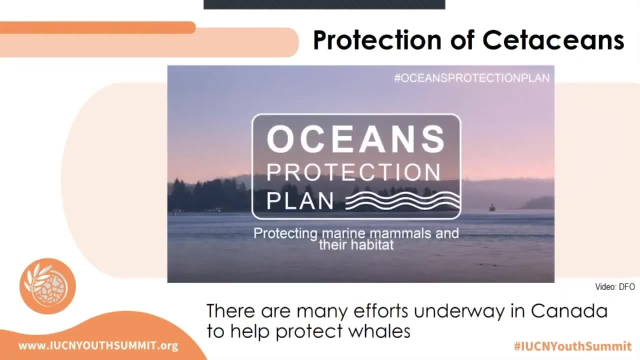 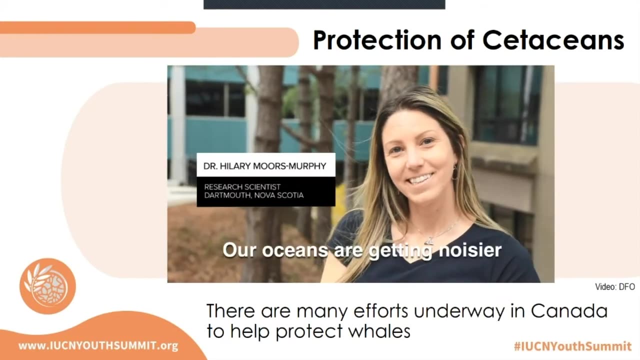 These are important threats that can negatively impact whales in our Canadian waters as well as internationally. In Canada, we have many different tools that can be used to help protect whales. This includes formal legislation that prohibits the killing, injuring, harming, harassing, disturbing, capturing or taking of whales. 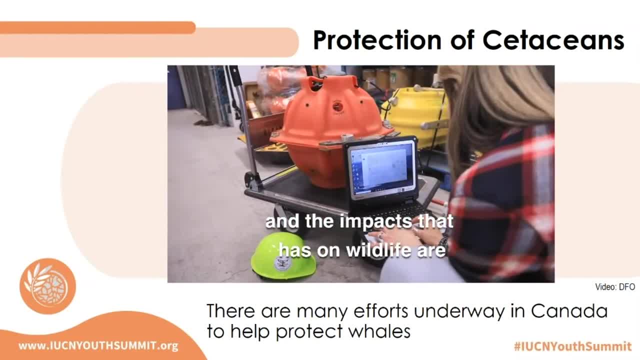 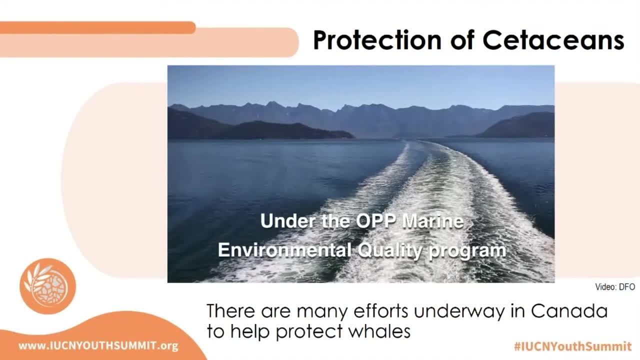 or destruction of their habitat. like our Fisheries Act, our Species at Risk Act and our Oceans Act, Designation of critical habitat for species at risk And establishment of marine protected areas and other similar conservation areas also help protect whales in Canada. 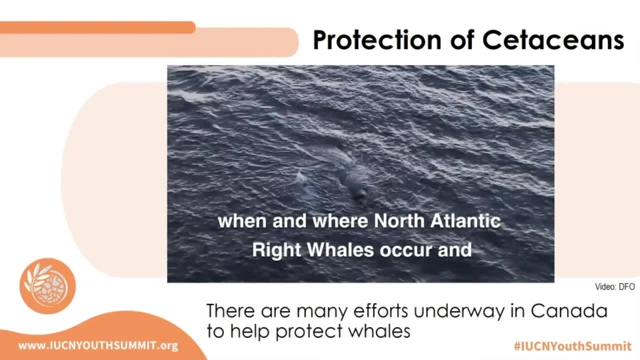 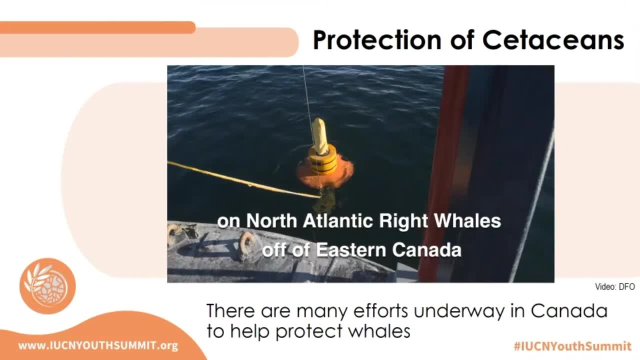 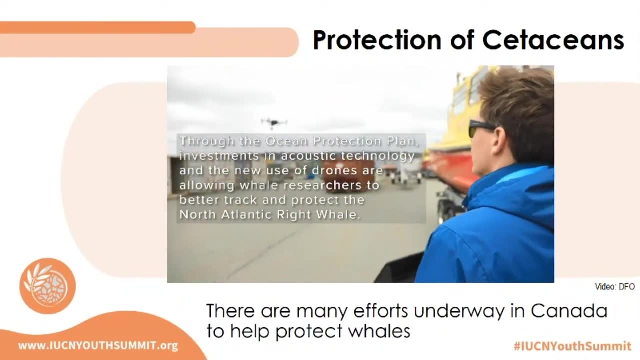 We have static or fixed, as well as dynamic or more flexible management measures in place for protection of whales, And, in addition to mandatory measures, we have voluntary measures, best practices and a number of guidelines out there aimed at decreasing the risk of human activities on whales. 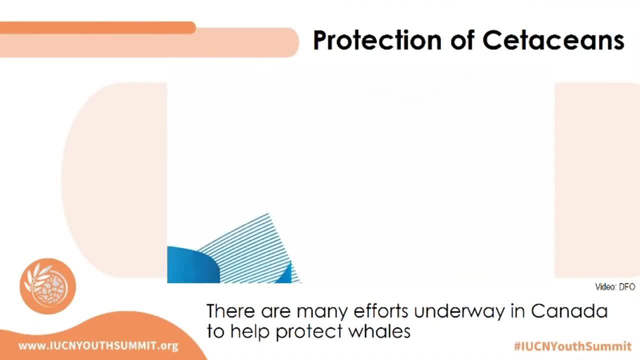 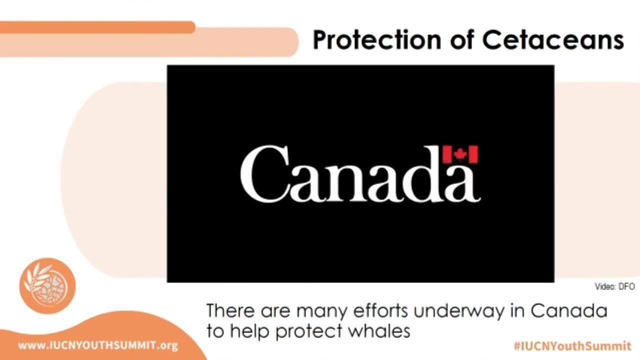 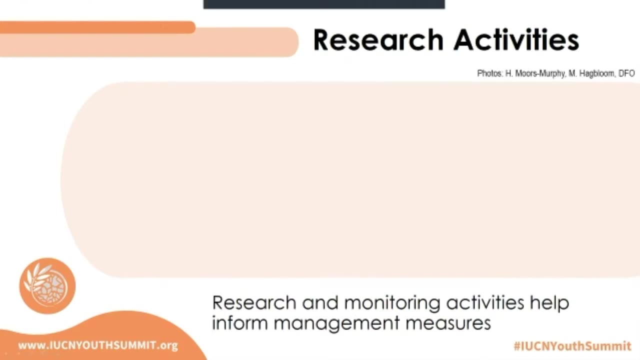 And we also have a number of research programs underway to help address threats to whales, Such as work being conducted as part of our Oceans Protection Plan, And that's some of the work that my team and I are doing as well, So this is where my work fits in. 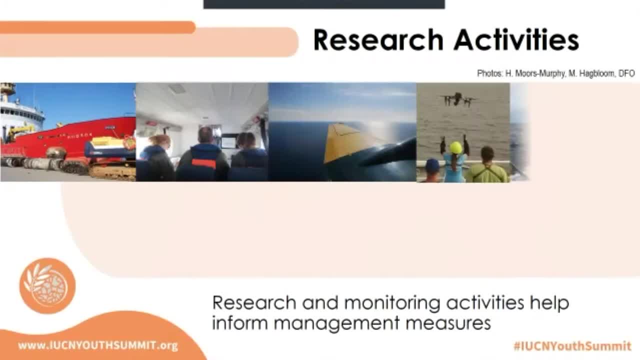 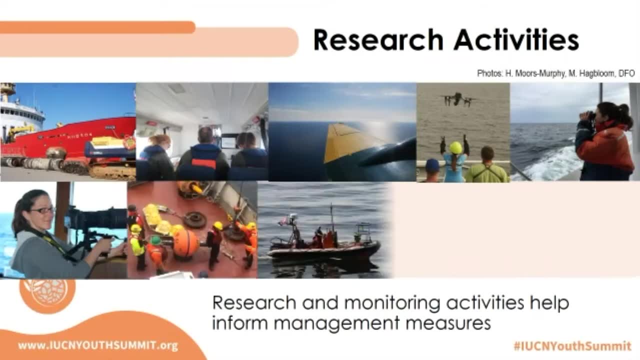 Research and monitoring activities can be used to help inform actions to reduce threats to whales, And there are so many different whale-related research activities being conducted in Canada by many, many different organizations, including Fisheries and Oceans. So the rest of this talk I'll highlight just some of the research and monitoring activities at Fisheries and Oceans. 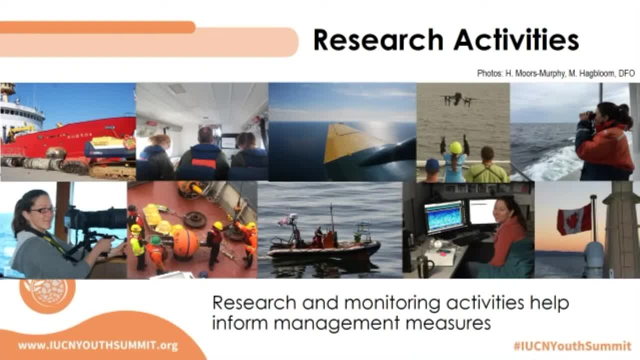 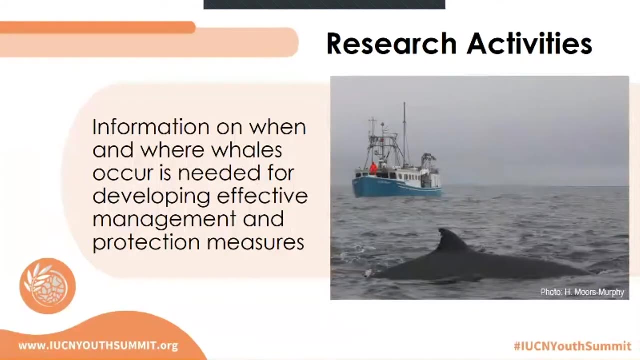 and in particular my team is involved with off of Eastern Canada that are being conducted to help support the protection of whales in our waters. So information on when and where whales occur throughout the year is important for understanding their distribution and habitat use. It's also important for assessing potential threats to populations. 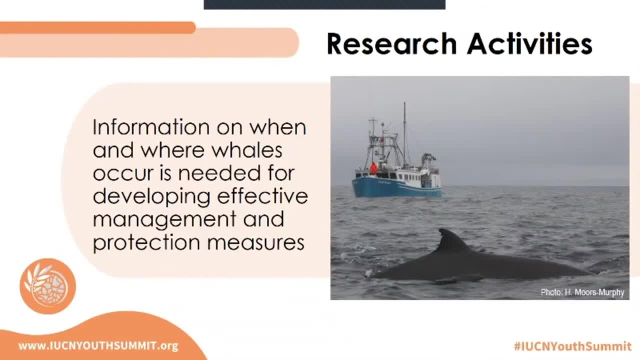 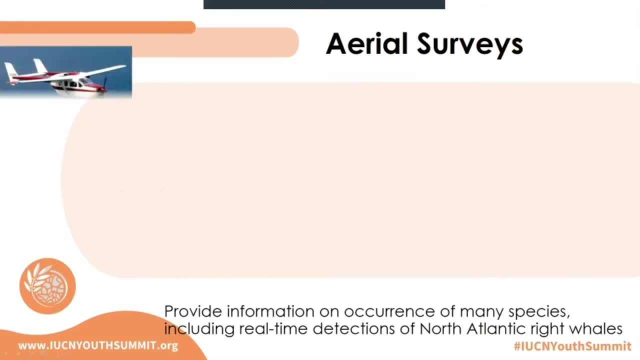 and developing effective management strategies and mitigation measures to protect individuals and populations. Aerial surveys are an important source of information on whale occurrence off Eastern Canada. Sightings of whales have been collected by trained re-mammal observers that have worked from a number of different aerial platforms. 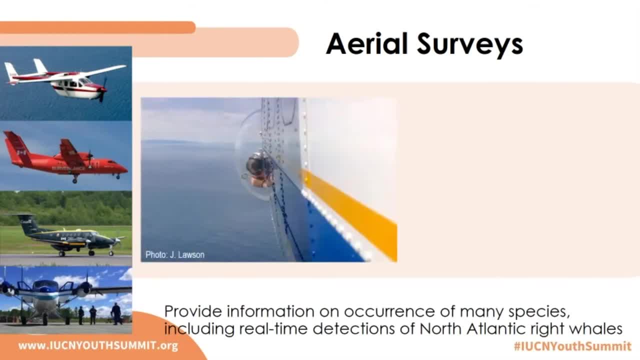 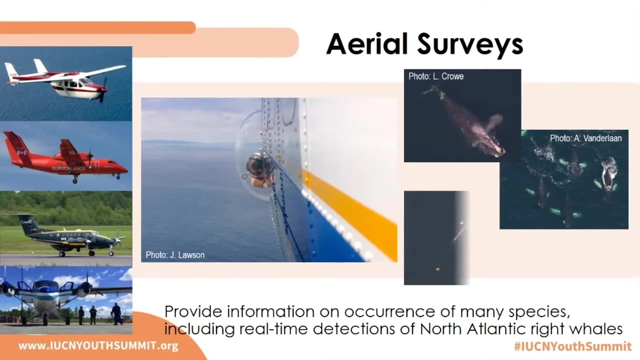 including those run by Fisheries and Oceans and Transport. Canada and even the United States National Oceanic and Atmospheric Administration, has assisted with whale survey work in our waters. Some of these planes are equipped with special bubble windows which observers can sit in, to allow for easier spotting and identification of whales from the plane. 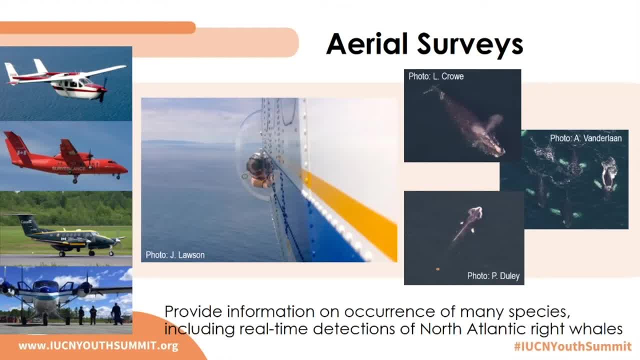 and I have a picture of that in the middle of my slide here, Because planes are fast. aerial surveys provide information on occurrence over broad spatial ranges and these surveys are particularly important for real-time surveys, real-time detection and monitoring of the highly endangered North Atlantic right whale off Eastern Canada. 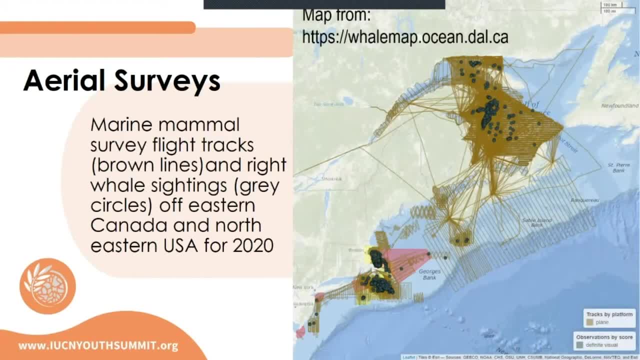 So over the past few years, whale aerial survey efforts have been increasing substantially off the coast of Eastern Canada, with well over a thousand hours flown by these various platforms in 2020 alone. And this map shows the aerial survey coverage and you can see the flight paths of the planes as these brown lines. 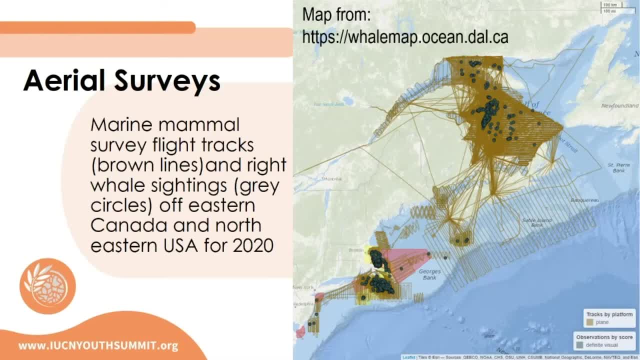 and the associated sightings of right whales, which are all the grey circles you see on this map for 2020 in both Eastern Canada and the Northeastern USA. So many of these right whale sightings in Canada resulted in fisheries closures and or vessel slowdowns to help protect right whales from entanglements in fishing gear and vessel strikes. 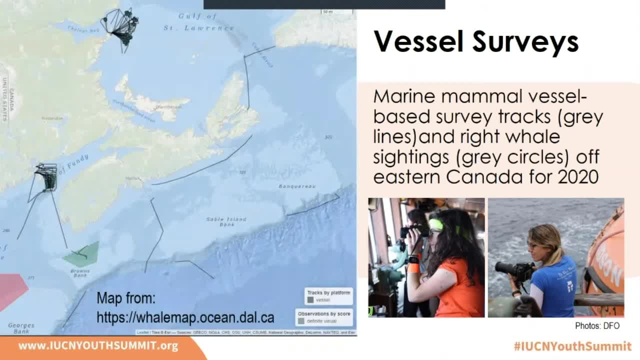 Similarly, vessel-based surveys conducted by trained marine mammal observers also provide information on whale occurrence, though, it takes a lot longer to cover ground in a boat, And this map is an example of some of the vessel-based work conducted in Atlantic Canada in 2020,. 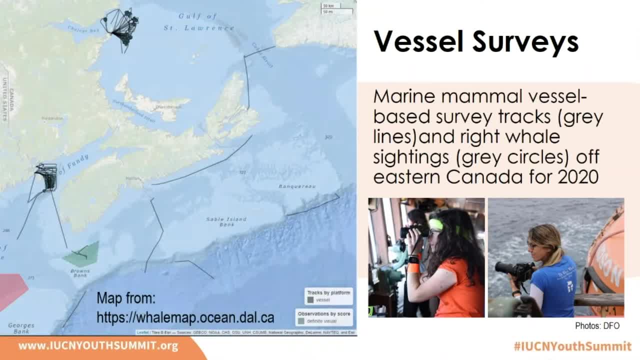 with vessel tracks shown as the grey lines that you see on the map, And these are just the vessel tracks when marine mammal observers were booking for whales And the grey circles are right whale sightings. So some of these sightings also resulted in management actions to protect right whales. 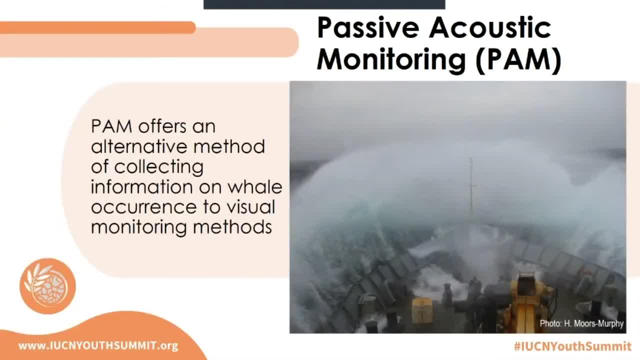 While vessel-based monitoring methods provide lots of information on whale occurrence, aerial and vessel-based surveys are limited to good weather conditions and sea states. So, as you can imagine, it can become quite challenging to collect data on whale presence during certain times of the year when you're out on a boat or up in a plane. 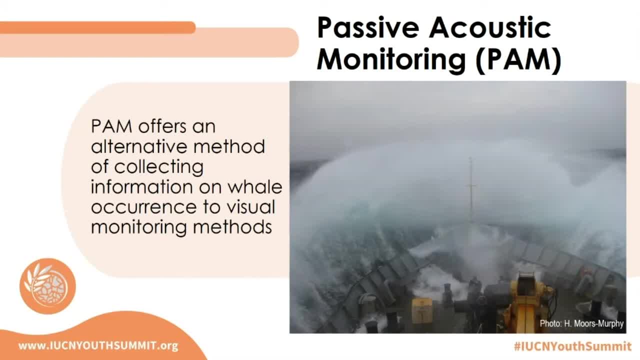 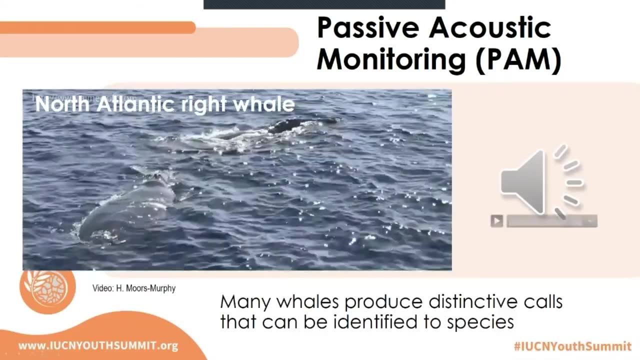 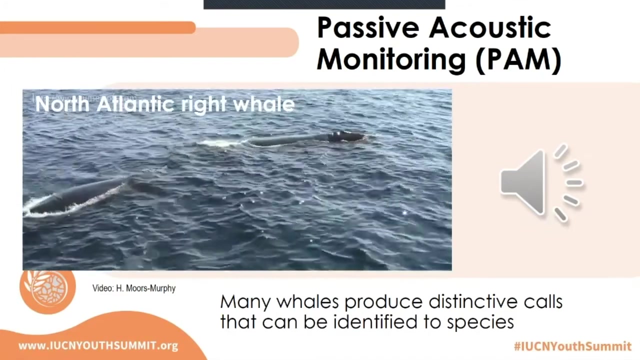 and particularly during winter months off eastern Canada. So passive acoustic monitoring or listening for whales, offers another way to collect information on whale occurrence throughout the year. So whales use sound for just about everything they do and most species are highly vocal. In many cases we can actually identify whale calls to the species level. 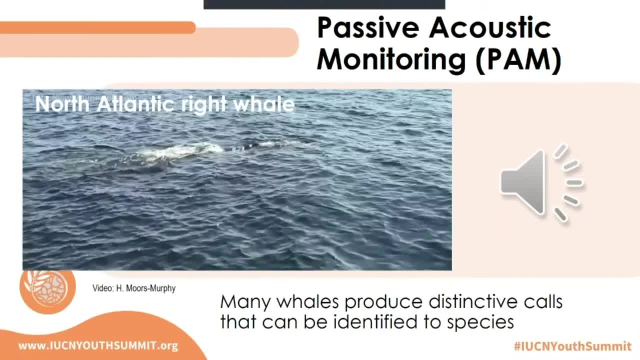 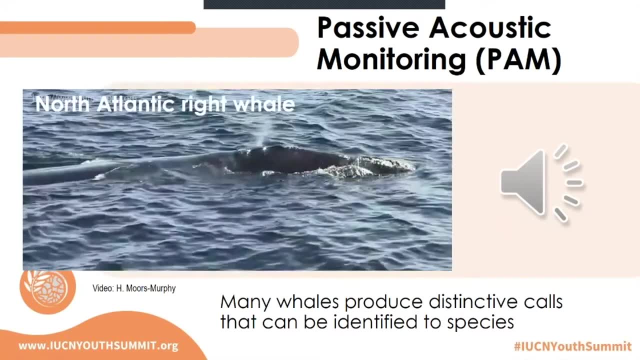 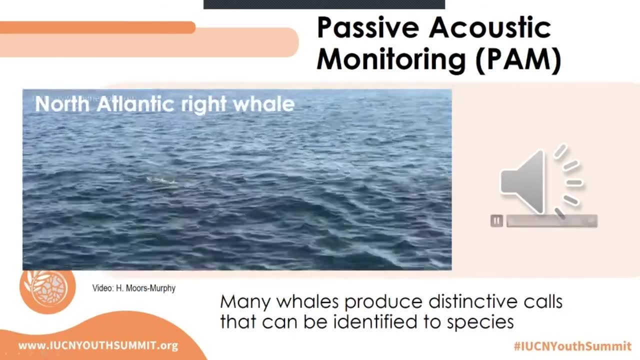 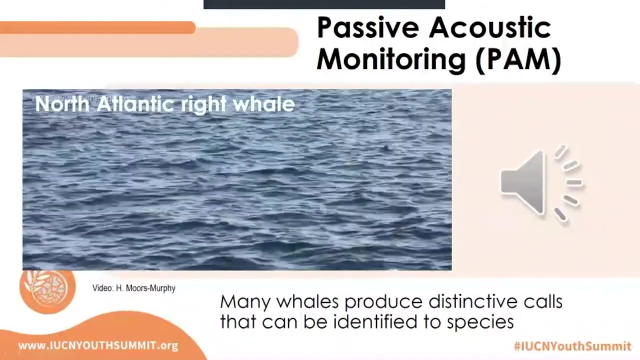 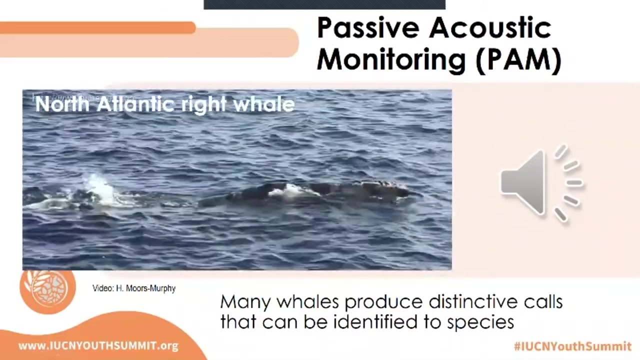 For example, I'm going to play for you now a stereotypical right whale call that's called an up call. And it's called an up call because it goes up in frequency, So it sounds a little bit like a whoop. And just out of curiosity, was anyone able to actually hear that sound clip? 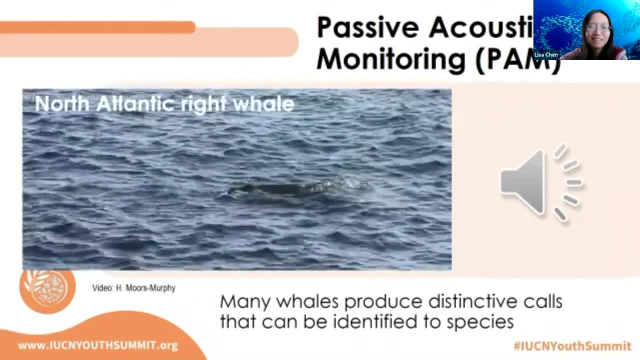 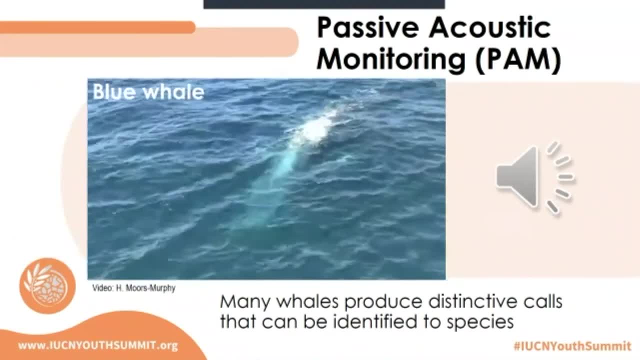 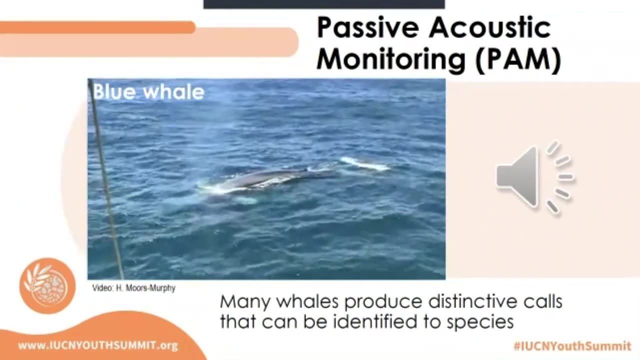 Yep, that was great. Okay, perfect. Now calls produced by other species. so I just played a right whale call. calls produced by other species, like these blue whale calls, sound quite different than the right whale calls, So this one you have to listen to very carefully. 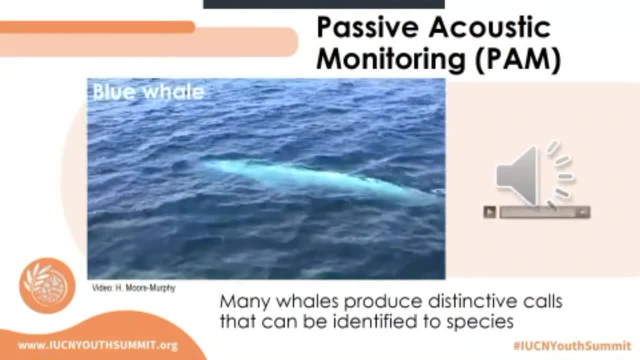 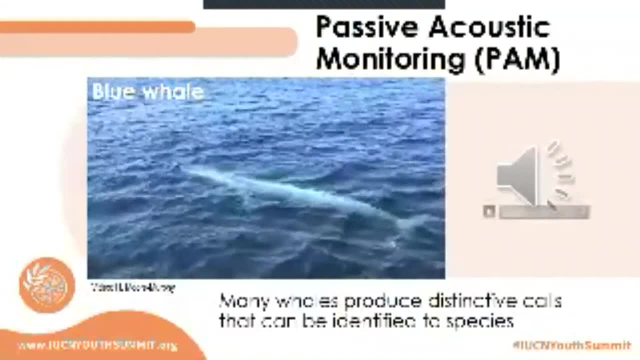 Because it's a very low frequency call, So I'm not sure.